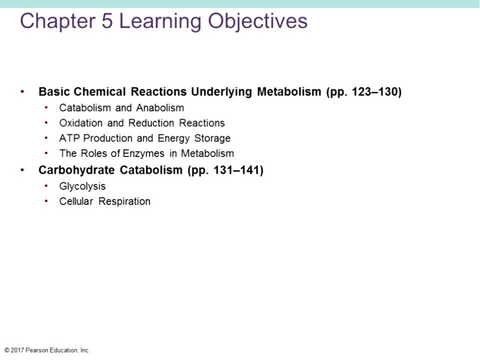 Hello everyone and welcome back to Microbiology. So today we're going to talk about microbial metabolism And I'll have to tell you guys something: That metabolism is actually one of my favorite topics to discuss ever, because it's so intricately detailed and it's so much. 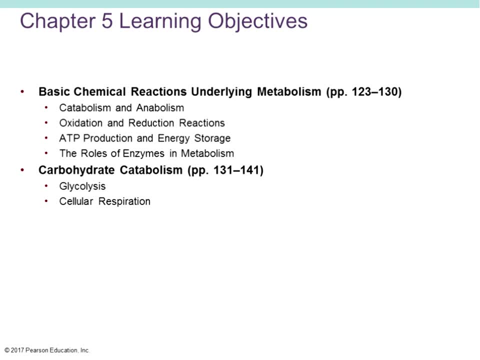 fun. There's so many little working parts to it, And guess what? It's happening inside of you right now. So, without any further ado, let's go ahead and jump on into it, As we've done for every other session that we've had. here are the learning objectives things. 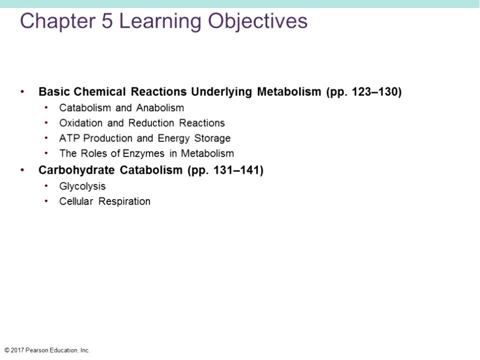 that I really want you to take from this session. This session is going to be in two parts, so be on the lookout for part two of it and make sure you watch both parts of the session. And I'm not going to read through all of these things, but in a nutshell, we're going to 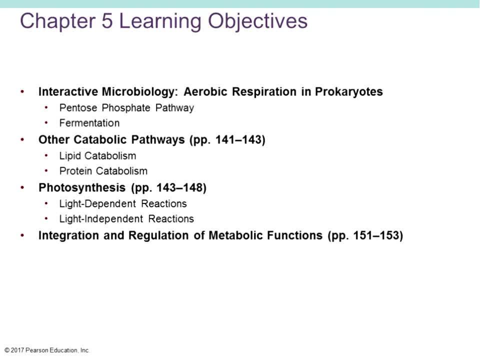 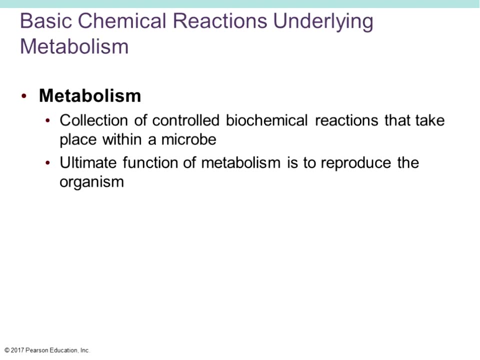 talk about metabolism, but it's going to be a little different than maybe the metabolism that you saw. So what is metabolism? Metabolism is just a collection of biochemical reactions that take place inside of a cell. In this case, the cell that we're talking about are microorganisms. 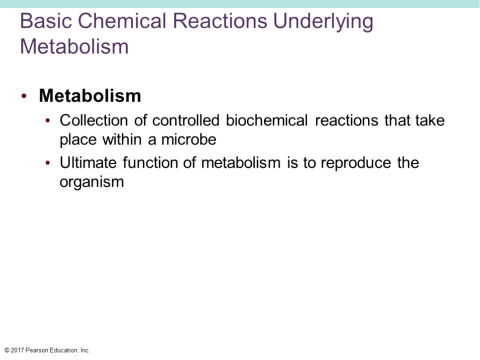 or microbes. All of the energy that is taken in via the form of the cell is going to be a form of foodstuffs, if you will, whether it's organic or inorganic, or even if it's sunlight energy that's converted into a different usable form. All of those reactions are considered. 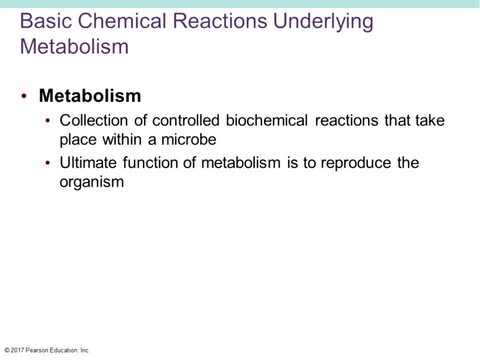 a part of metabolism. And then the other part of metabolism is the part where there are different proteins and carbohydrates or different end products that can be built up and made. So metabolism really consists of two integrative parts to it, two major integrative parts. 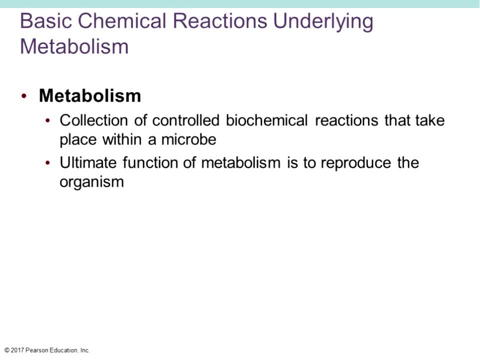 And those are catapults. The catapults are the metabolic properties and the anabolic properties. Catabolic properties are breaking things down to get energy out of it and you get these subunits that can be built back up in the anabolic properties into different types of macromolecules that 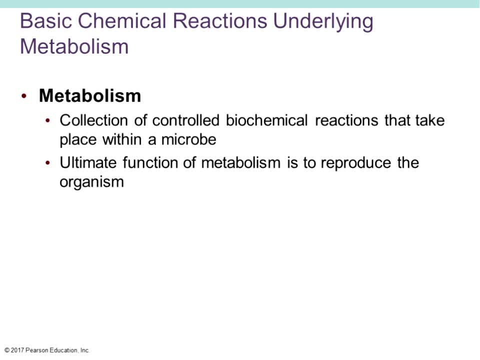 are useful for the cell. Now, if that kind of just went over your head right now and you're just like, what on earth is she talking about? I'm just kind of giving you a little teaser, a little preface, on what we're going to talk about, and we'll get the details of that as we go through this session. 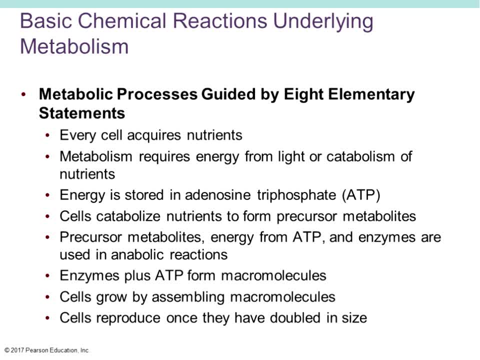 So metabolism is guided by eight pretty elementary or pretty basic statements. So those basic statements that guide metabolism are that? well, first of all, we know every cell has to acquire some sort of nutrients, so there are certain vitamins, macromolecules such as proteins and carbs or sugars that the cell is going to need in order to facilitate. 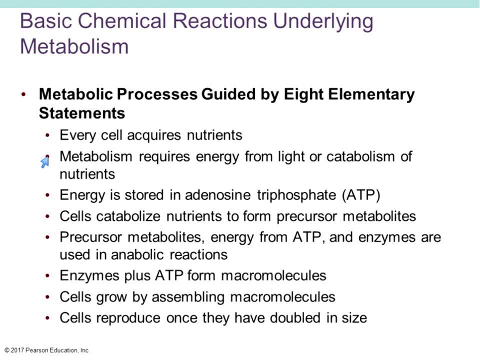 its growth, its life, whatever it needs to do. Another basic property is that metabolism requires energy from either light or the catabolism of those nutrients. Remember, when you see catabolism, I want you to think, breaking stuff down. So the 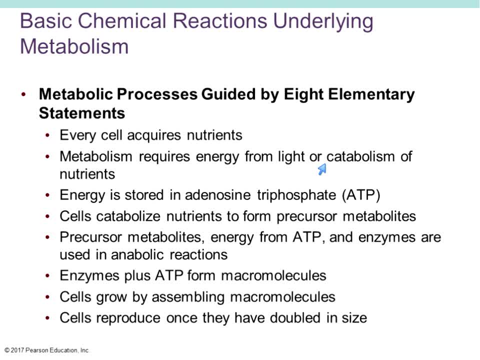 nutrients that you get, or the nutrients that a microbe gets, it's going to have to have the ability to break it down, And the way that microbes and yourselves can break things down is usually with the help of an enzyme. Enzymes help to speed. 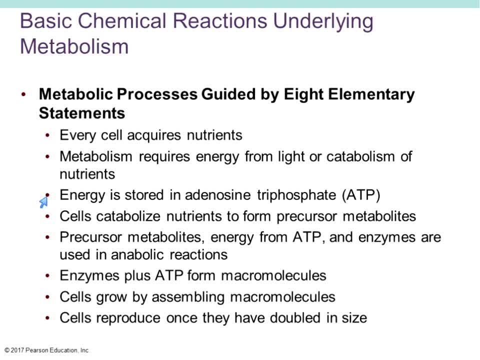 up that reaction of breaking something down and then getting the energy out of those bonds. The next basic statement is: well, energy is stored in the form of ATP or adenosine triphosphate. All of you guys have had an introductory biology. 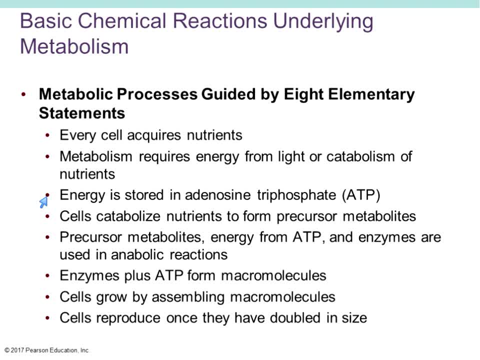 course, and you're all very familiar with the cellular currency that we call ATP, and that's how it powers your muscles, that's how it powers flagella, that's how it powers cilia, that's how it powers any type of energy requirement: Endocytosis, exocytosis. 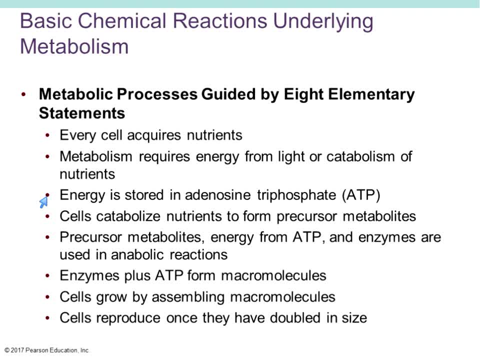 hyaluronic acid Communication. anything that requires energy in the cell is going to be powered by ATP. Cells can catabolize. and remember what did we say that says catabolize or catabolism? What basic term did we use to refer to that? Breaking something down to get energy out? 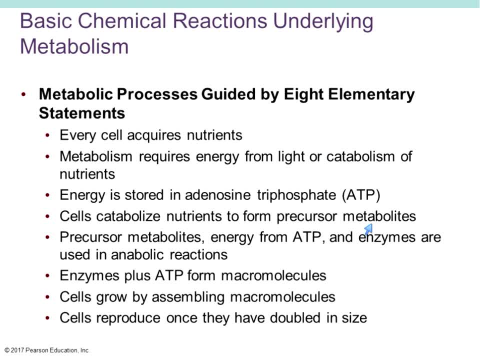 of it. So cells can break down nutrients to form precursor metabolites, And these precursor metabolites are going to be things such as the building blocks of the cell, the cells building blocks for proteins, which are amino acids, and the building blocks for carbohydrates. 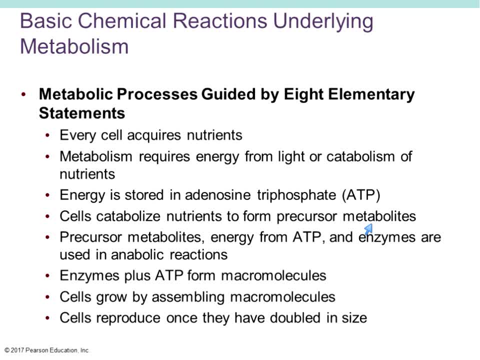 which are sugars, or the building blocks for nucleic acids, which are nucleotides. So there are different building blocks depending on what class of macromolecules we're talking about. Precursor metabolites, energy from ATP and enzymes are used in anabolic reactions. 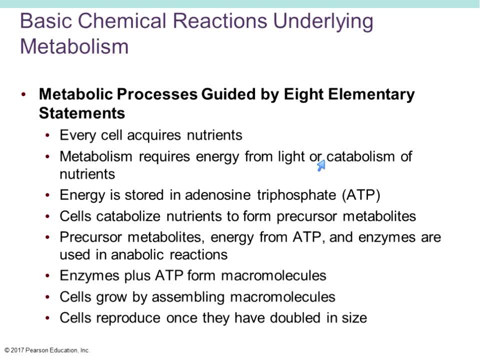 So anabolic reactions, this is where we're going to build things up. So in catabolism we're breaking things down and we get these intermediates or these subunits or metabolites. See, there are different terms that we can use to describe the exact same thing. So you, 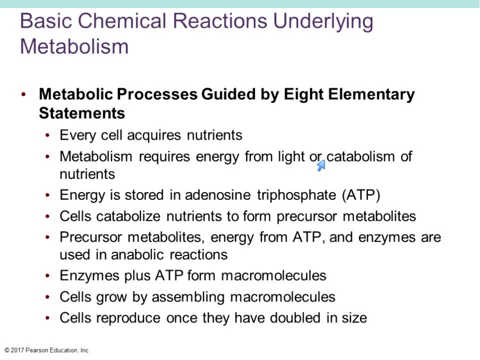 break things down in catabolism, you're going to get smaller building blocks from them and in that process of breaking things down to get those smaller building blocks, you're going to get some ATP or energy. You also have these enzymes, and remember enzymes. 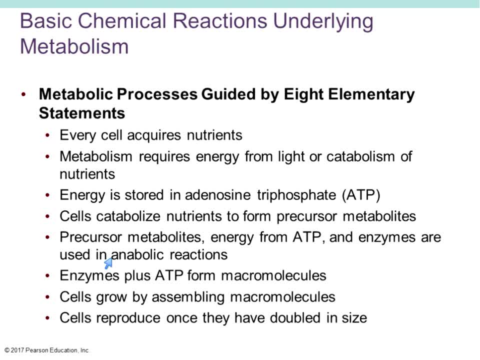 are catalysts. They can speed up the rate of a reaction. All of those things are going to be used in anabolic reactions. So what are these verbatim reactions? So they can actually make up anabolic reactions and we're going to need them in anabolic reactions to build up into something else. 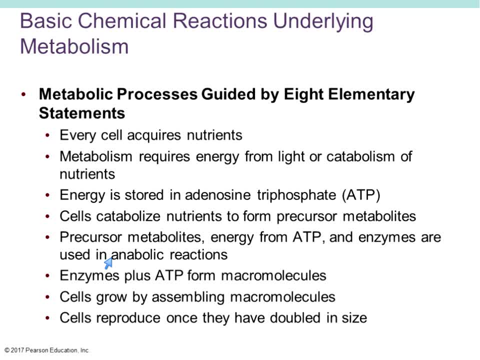 So there's going to be a building up. Remember, metabolism is two major steps. We have the breaking down portion of it we call catabolism, and then the building up, which is anabolism. Enzyme plus ATP form macromolecules. There are four classes of macromolecules, I'm sure. 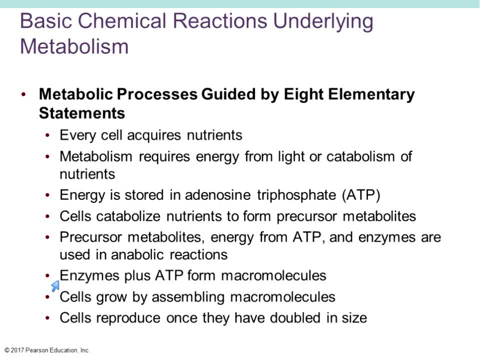 you're very familiar with. We have proteins, We have carbohydrates, we have nucleic acid And we have lipids. So those are our four classes of macromolecules. So just because- and let's just refer at this to your, your own life- So you ate an apple for breakfast, your body broke that apple down into the glucose. 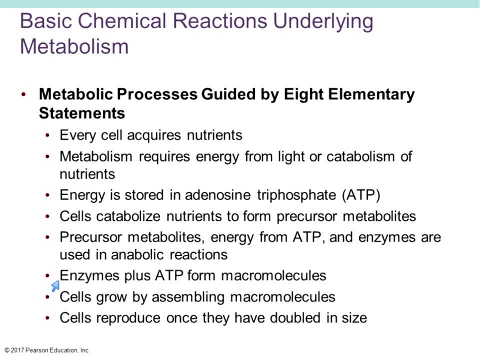 molecules that form the carbohydrate chains that make up your apple, and you also got energy out of it. Now you need to take that glucose and you need to turn it into a different type of macromolecule. You need to turn it into glycogen, which is a carbohydrate, in order to be stored. 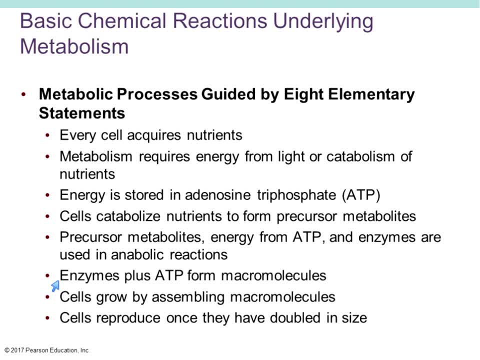 for your muscles. So you're going to take that glucose and you're going to hook it up with other glucose molecules and it will form glycogen or this macromolecule. Now, in order to build those bonds, we're going to have to invest some energy into it. So we're going to have to invest. 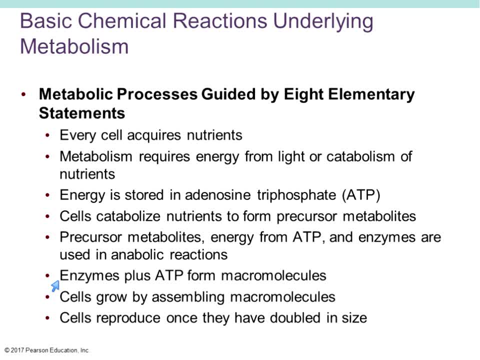 some ATP to link each of those glucose molecules together in order to make this glycogen that's used in your muscles. Prokaryotes, bacteria, microbes- they have the same sort of process that happens. They just may not necessarily be making glycogen like you are. They might be making. 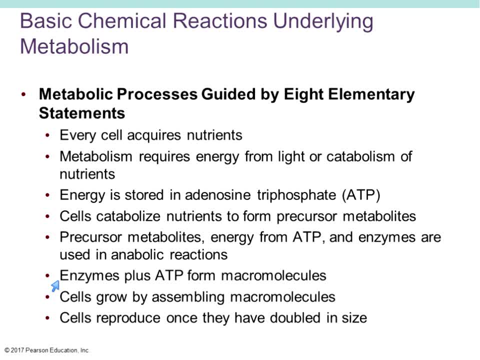 peptoglycan for their cell membranes. but the same principle still remains: that they have to take some sort of nutrient, break it down, get energy out of it, use some of that energy and the subunits from breaking down that foodstuff into a different type of macromolecule that is useful for the microbes So grow. 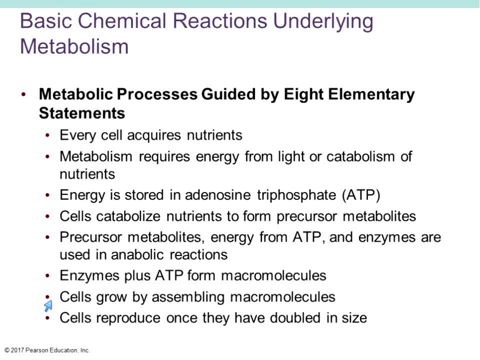 by assembling these macromolecules. Remember there are four classes: fats, carbs, nucleic acids and proteins. and cells reproduce once they have doubled in size. So the cells are able to, because that's really the underlying purpose for metabolism, you know, in an indirect. 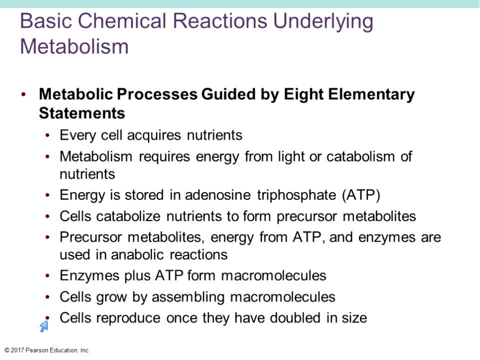 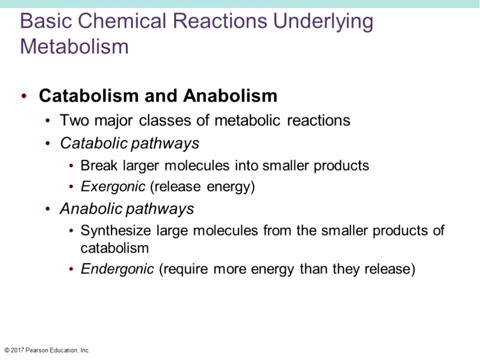 way is to make sure that this cell is able to put genes into the next generation and able to have progeny cells, the progeny microbes. So the two major classes of metabolic reactions anabolism and catabolism we have talked about quite frequently already and we're only on 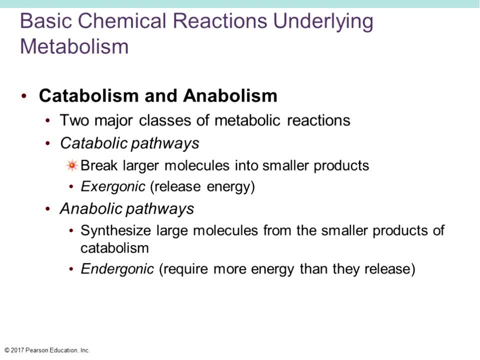 like you know, the sixth slide in here. So catabolic pathways, remember, break larger molecules into smaller products. It is going to be a release of energy. So we see that we have here EX. if you see the exit sign of the door or a room, that means you're leaving out. Exocytosis is a 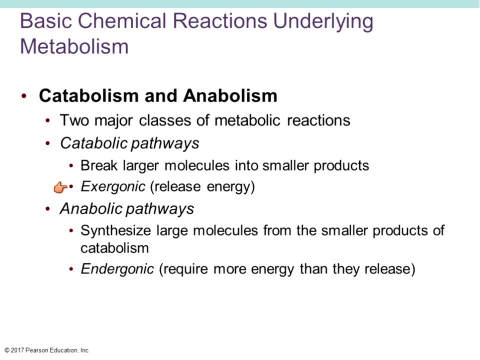 process where molecules are leaving out of the cell. So exergonic reactions are going to have the exit of energy, So catabolic reactions are going to release energy- we call that an exergonic reaction- and they break down larger macromolecules like proteins, carbs, lipids and nucleic acids. 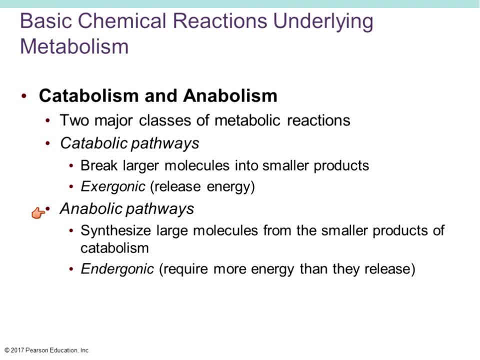 into smaller products. On the other side of that, we have anabolic pathways In anabolism. we're going to take those smaller products and we're going to synthesize larger or make. whenever we're synthesizing something, we're building or making something. So we're going. 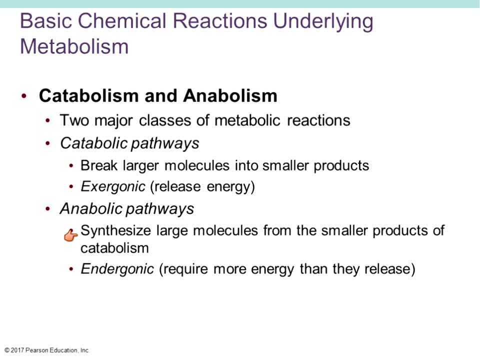 to make a larger molecule from that, those smaller building blocks, Because we have to invest energy into this process. we would call this an endergonic reaction. So, like endocytosis, things are going to be coming in. An easy way to remember. an anabolic pathway is building. 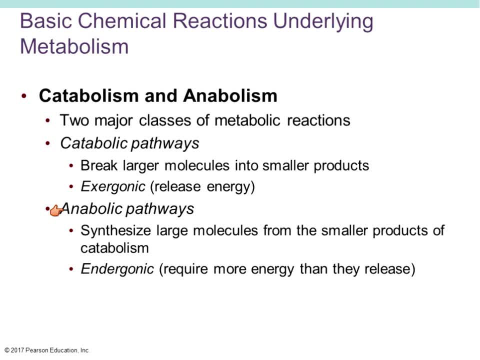 things up. Think about anabolic steroids. When you're taking anabolic steroids, are you breaking down muscles or are you building up muscles? So anabolism is the building up of things. In this case, we're building up macromolecules from these smaller subunits. 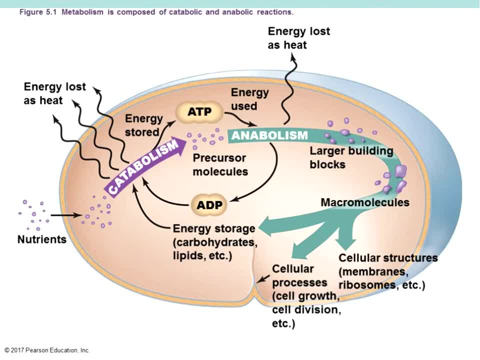 or smaller products, and that's going to require the use of energy. So here we have a nice little pretty cell where all of the stuff is going on. We have our catabolism, So we have the nutrients that are coming in. So whatever those nutrients. 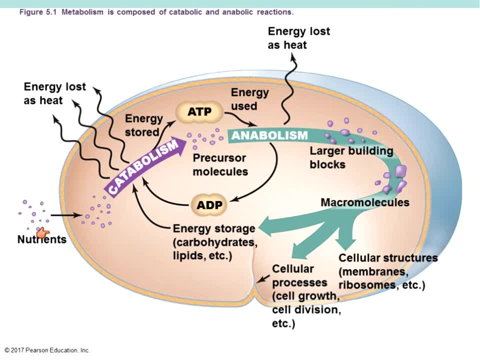 are proteins, carbs, lipids, nucleic acids only do a whole lot of energy, but we could put them in that category. But those macromolecules. Then we have them broken down. When we break them down, We're going to get some of the energy that's stored in them and we get that in a usable form of ATP. 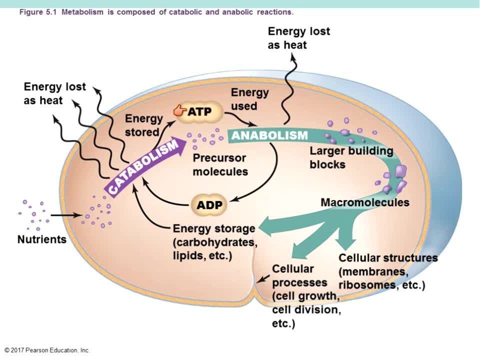 Now we don't get to use all 100% of that energy that's stored in the nutrients that we broke down, but some of it's going to be lost off as heat to the atmosphere. So that's what these wavy lines signify: that you know a little bit of it is lost off as heat. 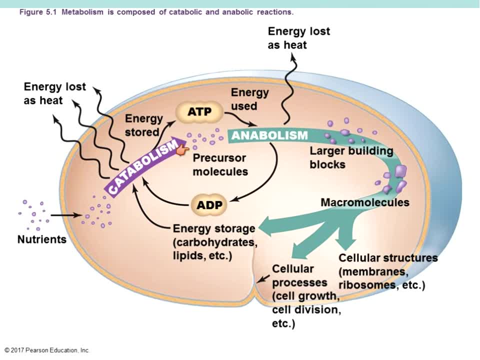 Then we can use that ATP plus those molecules that built up the nutrients. so we've broken them down into these little guys here and we can build them up in an anabolic property, And much the same way that we lost a little heat in catabolism. 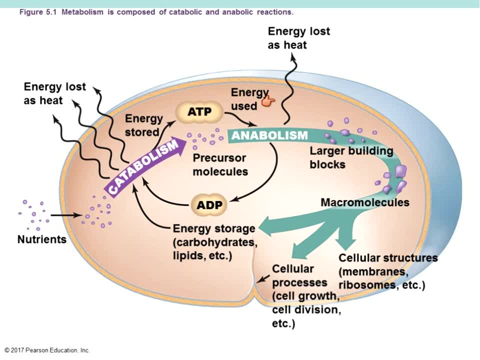 well, there's just a little bit of heat. not nearly as much as when we break things down, But there is some small amount of heat- notice fewer arrows in here- some small amount of heat that is lost to the environment in building up. 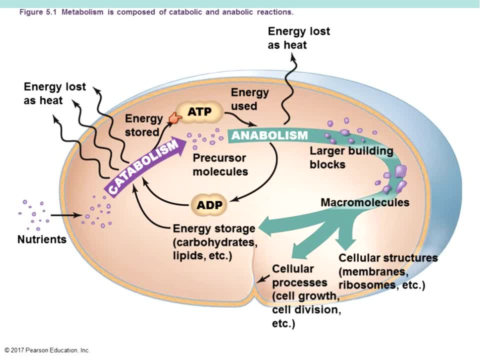 So these precursors plus the ATP in an anabolic reaction are going to- or also called endergonic reactions- build these larger molecules. These larger molecules are those macromolecules that can be used for various purposes. They can create different activities to build cellular structures, things like membranes. 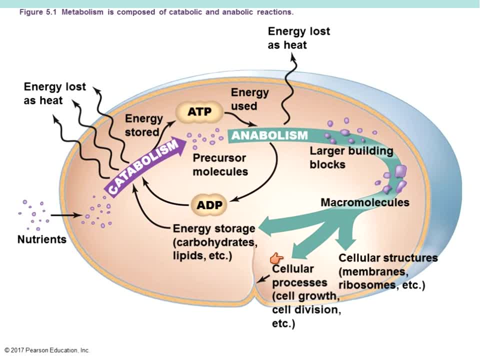 ribosomes, flagella also for cell growth and division, different cellular processes that happen within the cell and then even for some energy storage. So we talked about inclusions and how those inclusions are. different types of energy storage have energy storage capabilities. 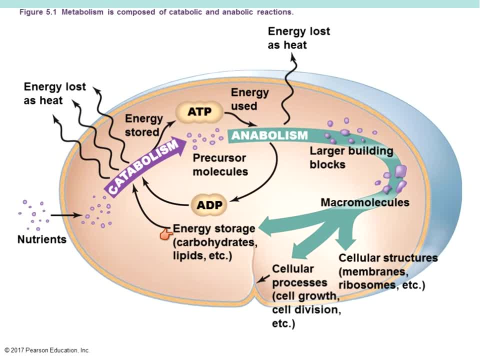 Most of the inclusions are storing some type of energy. So in a rainy day, if you get in a pinch and you can't get any nutrients right away, then you can break down those energy storages in order to get ATP or energy. 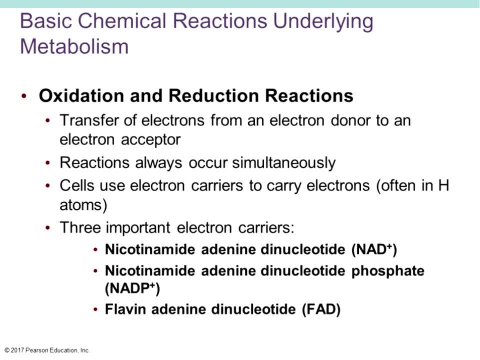 So the basic chemical reactions that are involved in metabolism. so far, a lot of this should seem pretty familiar that you've seen this before, you've talked about it before in an introductory biology class. Nothing that we said up to this point has any is different from eukaryotic cells. 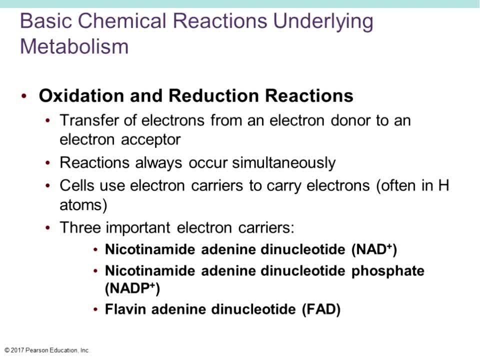 These proteas will do the exact same thing. So we're still continuing with that theme. that these prolatic cells will still conduct the same sort of base activity, So we'll continue with that theme. metabolic reaction: so when we talk about these anabolic and these catabolic, 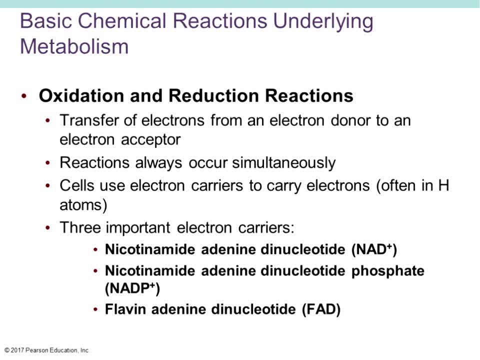 reactions. we're going a little bit deeper into this discussion and what we're really discussing: our oxidation reduction reaction. so so far we've just said: nutrients come in, they're broken down through catabolism and you get these smaller building blocks and you get some ATP out of it and those smaller 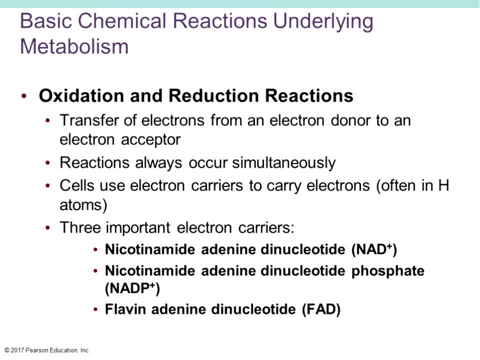 building blocks, or smaller products can be built up into larger products and anabolic reactions, and those larger products can be used to carry out various different functions for activities for the cells. Perfect, now we're going to see more detailed exactly how those things happen, and they happen through oxidation and reduction reactions. oxidation: it's 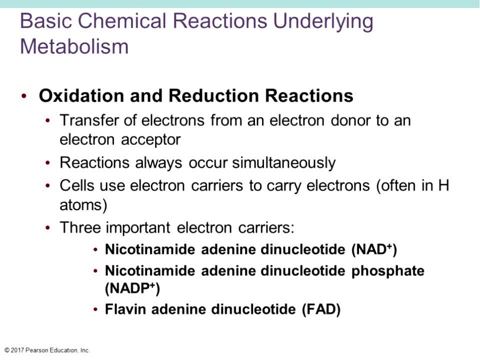 always going to be the laws of electrons and hydrogen. so an easy way to remember this is: oil. oxidation is loss, and reduction is the sector in where choice occurs: gain of electrons and hydrogen. So an easy way to remember that is: rig, oil rig. So oxidation, loss of electrons and hydrogen. 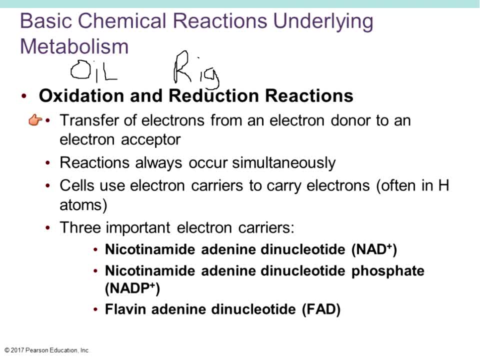 and reduction is a gaining of them. So really, another way to refer to that is that it's a transfer of electrons from the donor to the receiver. Oxidation and reduction reactions always happen simultaneously and that's why we just call them redox reactions, So it's just another. 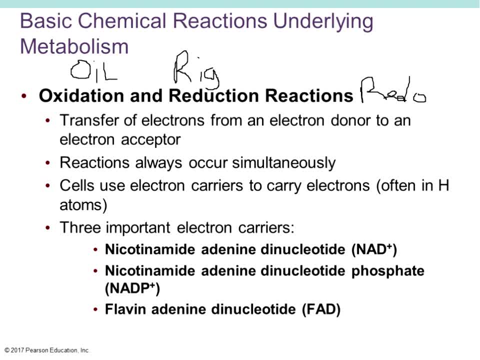 way to say that It's rig for reduction and ox for oxidation. Where one's losing, one's gaining. We use electron carriers to carry these electrons, and usually they're hydrogen atoms. so that's why I said the loss of hydrogen and electrons. 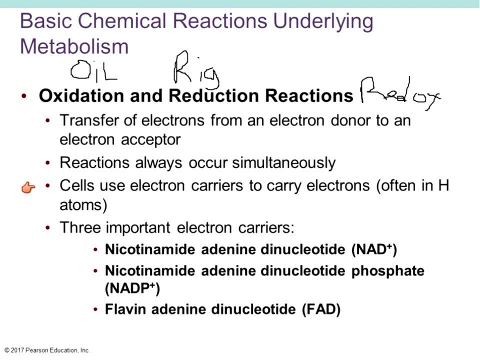 They don't just electrons just float willy nilly all the time And these reactions, they're going to be attached to hydrogen ions And there are three important electron carriers that we are going to discuss at length throughout this semester and especially throughout this chapter. 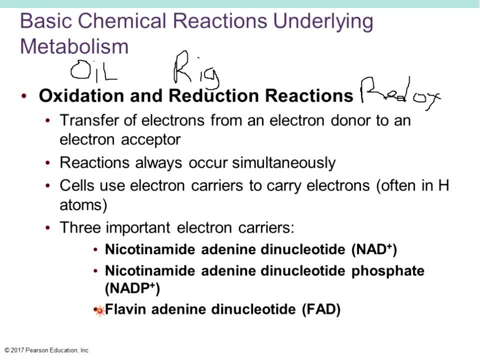 NAD, NADP and FAD. So make sure- and they're so important that I am going to even take the time out to highlight them so that you remember- Nicotinamide adenine dinucleotide and nicotinamide adenine dinucleotide phosphate. 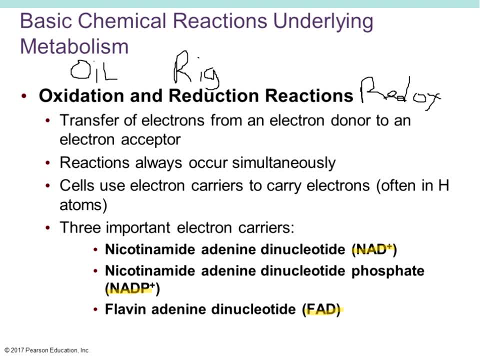 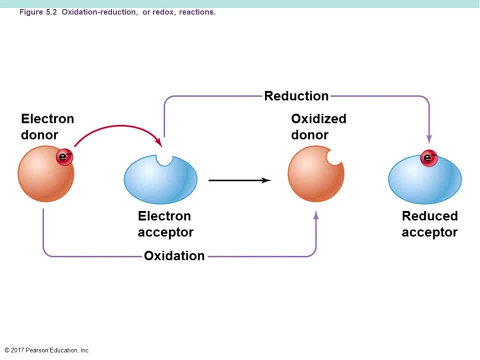 and flavin adenine dinucleotide. You don't have to know their full names, just know their initials. So here's a pretty picture of a redox reaction taking place. We have our electron donor and it's giving up its electron to the electron receiver, or acceptor. 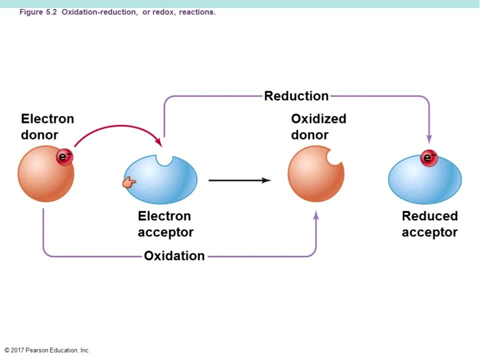 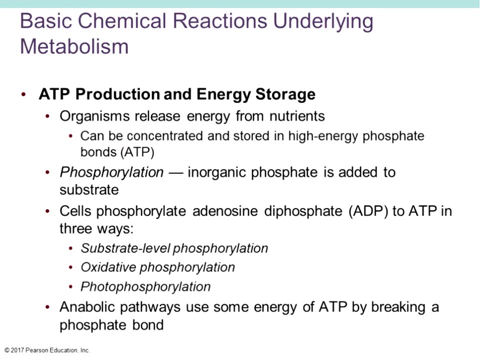 So since it lost its electron, we say that this molecule has been oxidized. Since this blue molecule is gaining an electron, we say that it's been reduced. Now that oxidation and reduction a lot of times is going to generate in the production of ATP and definitely 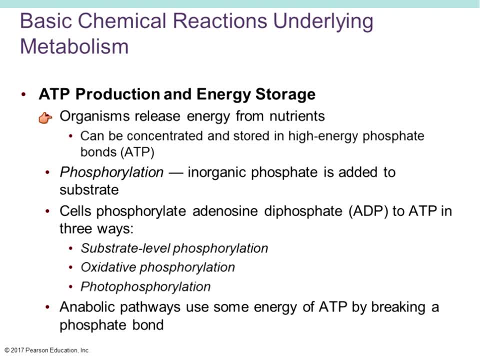 some energy storage. So organisms are going to release energy from their nutrients. through what kind of reactions? Catabolic or anabolic reactions? And also an important note to make is that oxidation and reduction reactions are not just relegated to catabolism. 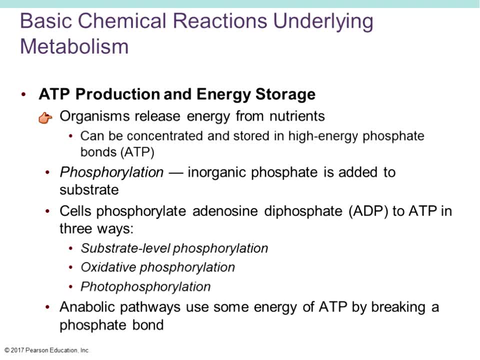 They're also going to be part of anabolism as well. So we see redox reactions on all parts of this process that we're talking about called metabolism. So ATP can be concentrated and stored in high energy, or energy can be concentrated and stored in high energy phosphate bonds. 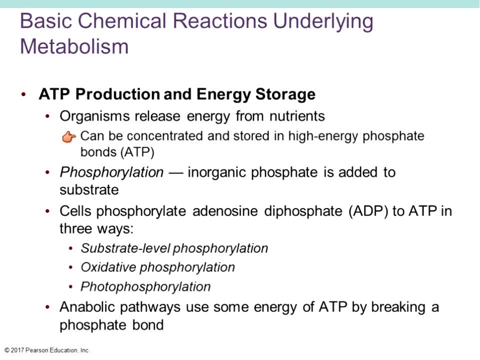 So if we put a phosphate at PO4- and if we put three phosphates- adenosine, tri-, tri- three phosphates together, there's a very stressful bond that's placed on that second and third phosphate because you have three negative charges that are right next to one another When we break the bond in that third. 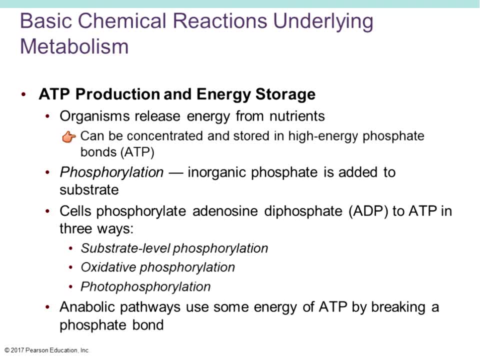 phosphate group. that's where that explosion of energy comes from. If we have an adenosine diphosphate and lost one of its phosphates off, we have this explosion of energy that was used for all these different things in the cell. we can put another phosphate on there And that process of 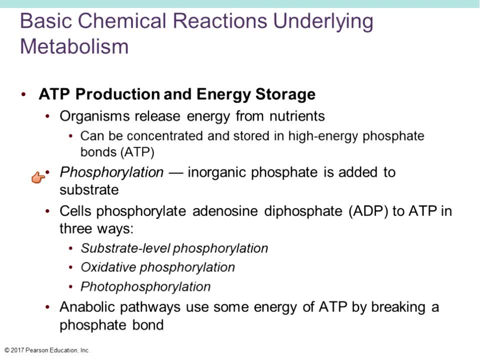 sticking another phosphate onto ADP or adenosine di-, two phosphates to make ATP-adenosine tri-, three phosphates, is called phosphorylation. Phosphorylation is a process by which a phosphate is just added to something, So you add. 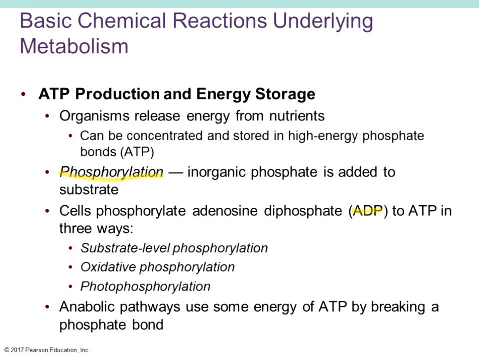 a phosphate to it, it's been phosphorylated. Now there are three different ways that we can convert ADP to ATP via this phosphorylation, And there's substrate-level phosphorylation, which is going to require the use of a substrate and an enzyme Oxidative. 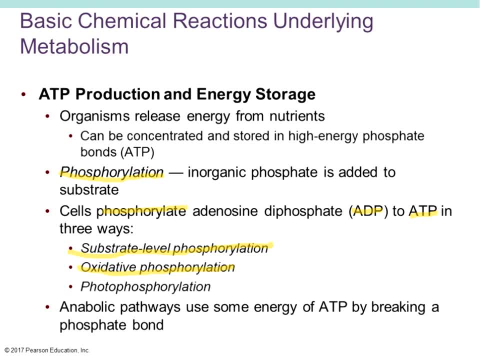 phosphorylation, which is a much larger process than an oxidative phosphorylation. We get to, basically, we go through all three stages of cellular respiration- and this is a more in-depth process that we're going to talk about in this chapter as well- And then we have photophosphorylation. 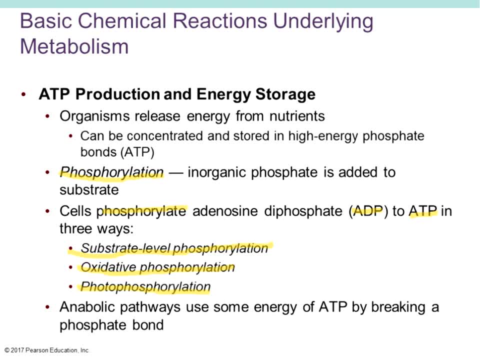 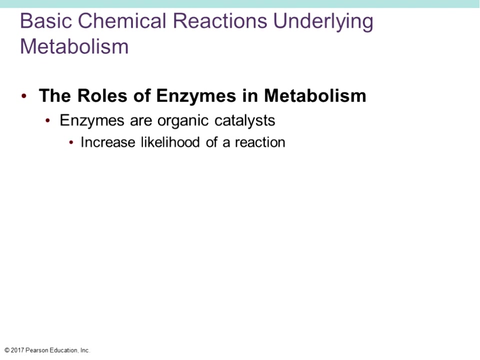 Photos meaning white cells. Think photosynthesis as a method of phosphorylation or as a process in which photophosphorylation can happen. Antibiotic pathways use some energy of ATP by breaking a phosphate bond. So that happens, but it's just some of it And it's usually to kind of start things, get things rolling. 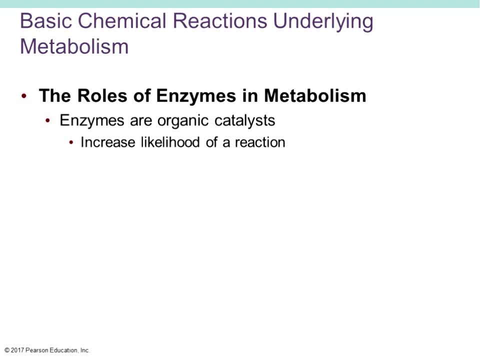 So enzymes are biological catalysts and enzymes help to reduce the rate of or speed up the rate of reaction by reducing the activation energy required to get that reaction to start. So when we have enzymes present it's going to increase the likelihood of that reaction. 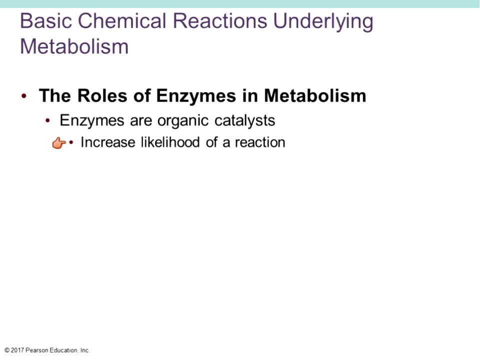 taking place. So these reactions probably would take place on their own, but they would take place at such a slow rate and the process would be so slow that life as we know it would cease to exist. So these enzymes help to reduce the amount of energy that's needed to get the reaction to start. 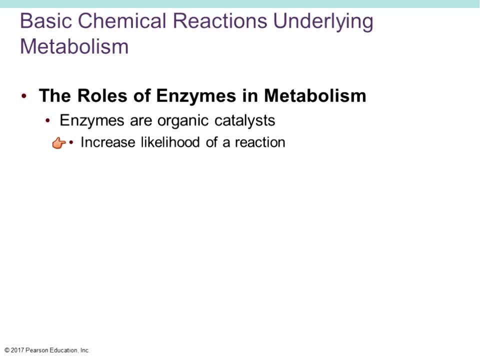 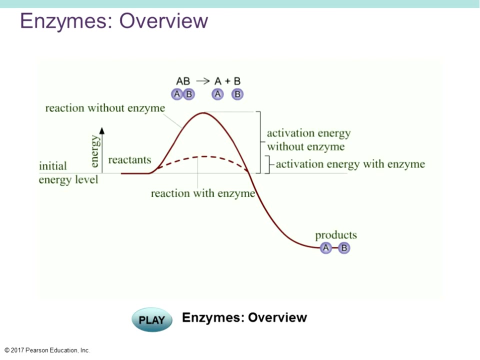 So since there's less energy that's required, then that process can happen faster, And this is very important for all of metabolism, but specifically important for substrate level phosphorylation. And what was phosphorylation? again, Just adding a phosphate group onto something, And notably phosphorylating ADP, to turn it into 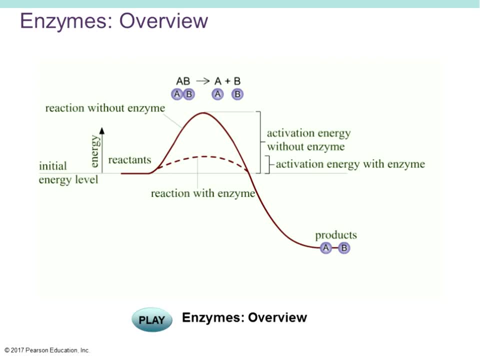 ATP for usable energy. So here we have a picture of enzymatic activity and just kind of an overview of this enzymatic activity. So if we have these two reactions that we want to take place, So we have this AB molecule that we want to convert. 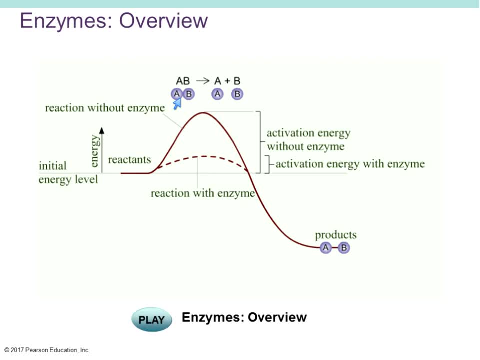 into an A molecule and a B molecule. We want to break this bond between the A and the B Much the same way that we would be breaking bonds between two glucose molecules in a catabolic property. Now, once again, keep in mind, although we've been using catabolism as an example, that is, 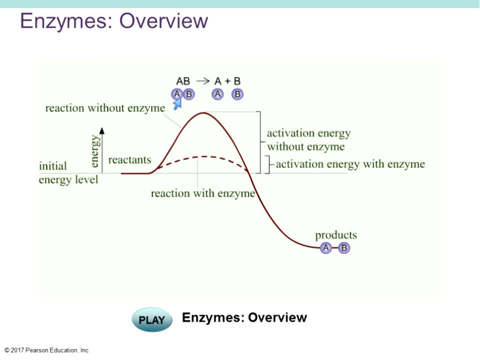 not the only part of metabolism that's going to require enzymes. So not only do you need enzymes, or is it nice to have enzymes to break bonds? it's also nice to have enzymes to build bonds as well, So we can see the same thing happening on the. 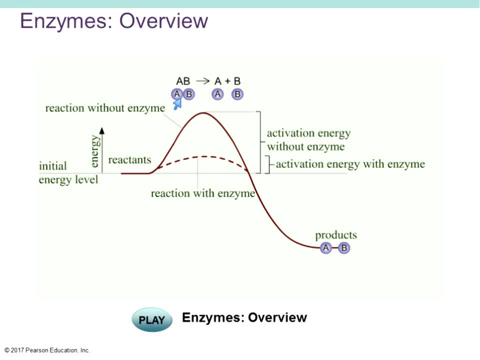 anabolism scale of all this. I just wanted to point that out to you guys so you won't think that enzymes are only catabolism. So in this case we want to break this bond here Now, if we don't have any. 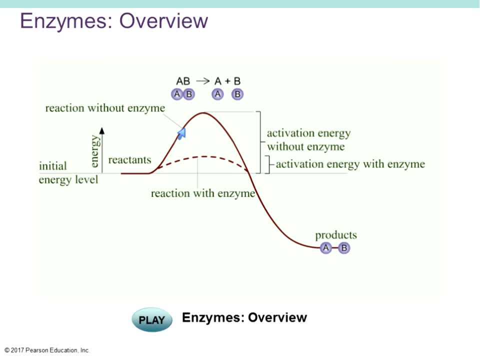 enzymes, we're going to have to use much more energy in order to get that process to take place, in order to activate these bonds to be broken, to get our products A and our products B. If we have an enzyme that's present, that's denoted by this dashed line, then notice. 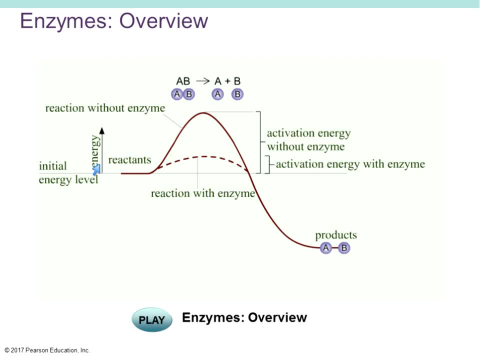 how there's a lot less energy that's required, So that activation energy is going to be much, much smaller. It's not going to take as long, It's not going to be as trying to get this reaction to take place. It speeds up this reaction, speeds up the rate of this reaction because there's 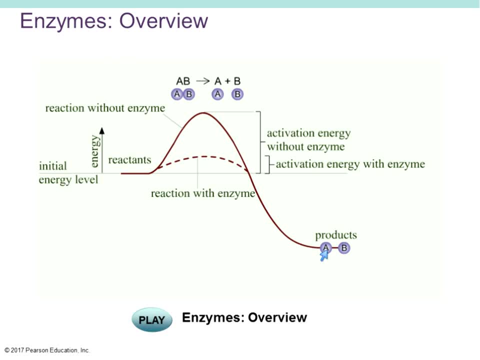 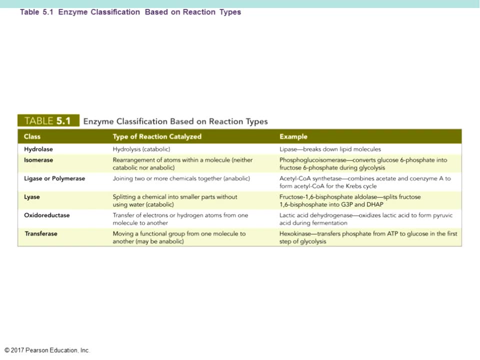 less energy that's going to have to be used in order to break this AB molecule into the products of A and B. So some enzymes can be classified based on the types of reactions. What I do want you to notice is that, for most of the enzymes that we're going to talk about- in fact, I think, all of the enzymes that we 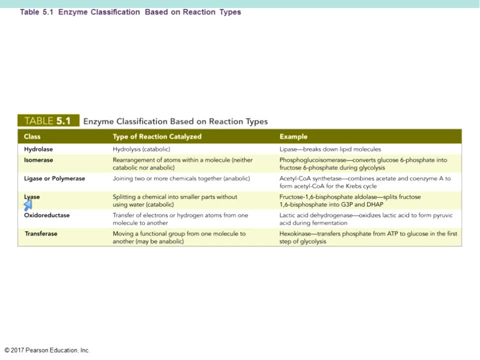 talked about in an intro, micro class- are going to end in ASE, So if you see something ending in ASE, that's a good indication that this is probably some sort of enzyme. So we have hydrolases that are going to use hydrolysis, which is part of a catabolic mechanism, and an example: 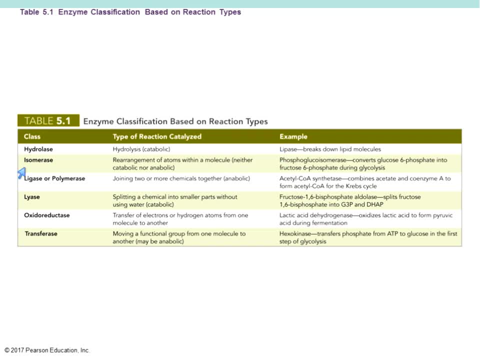 of that would be lipase that breaks down lipid molecules. Isomerases are going to rearrange the atoms and it's really not classified as either anabolic or catabolic. they're just kind of rearranging things. A good example would be glucose and fructose. They have the same 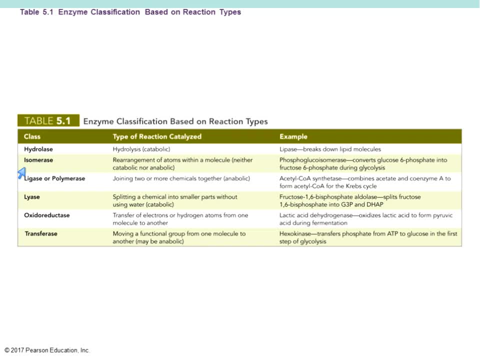 chemical structure to them, but their same molecular structure, but their chemical structure is different, where the carbonyl group is changed from primary to the second carbon between glucose and fructose. There was way more information than you asked for today, but the point is that you can rearrange the atoms. 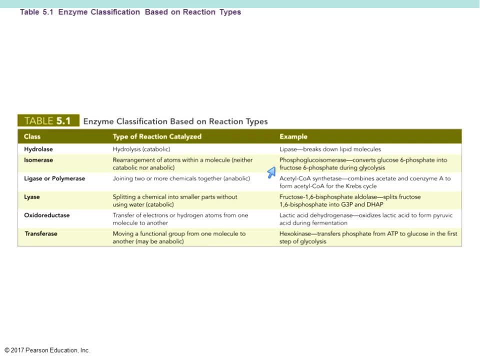 So actually that's a great example that they've used here. so phosphoblucoisomerase converts glucose 6-phosphate into fructose 6-phosphate. in glycolysis, Ligases, or polymerases, are going to join things together, usually in anabolic. 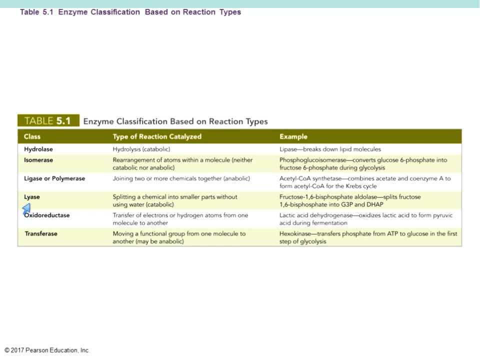 we're joining building up Liases, not ligases, but liases are going to split things into smaller products without using water, as we did for hydrolases here. so that's catabolic. Octoreductases are going to transfer electrons. 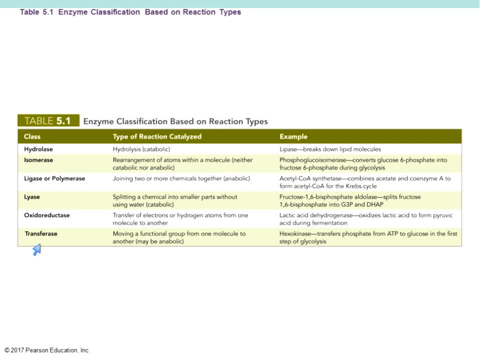 or hydrogens from one molecule to another, and then transferases are going to move functional groups like the carbonyl, sulfo, sulfohydryl, carboxyl- any of those six functional groups- from one molecule to the next. 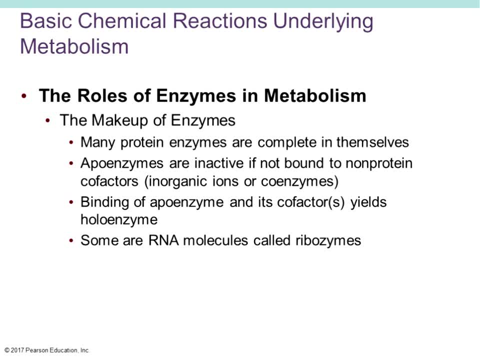 Okay So the role of enzymes in metabolism. we've already kind of established that they help to speed up the rate of the reaction by reducing the activation energy. The way that enzymes are made is that they're just basically proteins, So an enzyme is a protein, Every enzyme. 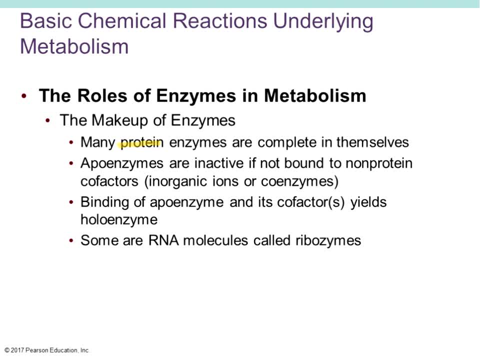 you ever come into contact with is a protein, but not all proteins are enzymes. So many enzymes or protein enzymes are complete all by themselves. Some of them, on the other hand, need another portion to them. So an apple enzyme is an inactive part of the enzyme. that's not going to actually 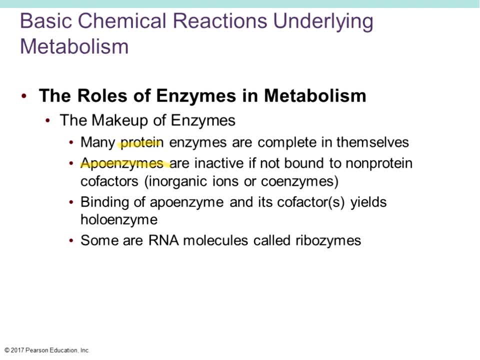 work unless it's bound to something else. So apple enzymes are inactive if they're not bound to a non-protein cofactor such as different types of ions or coenzymes. So binding of apple enzymes and cofactors. so together this guy. 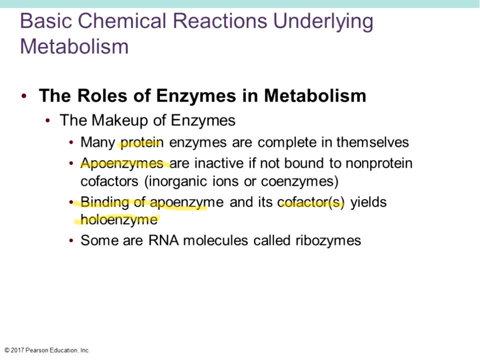 plus one of the cofactors, which could be inorganic ions or coenzymes, are going to give you a whole or a hollow enzyme. Some enzymes make up our RNA molecules, and if it's an RNA molecule that's acting as an enzyme, then we call it a ribosome. This is going to be. 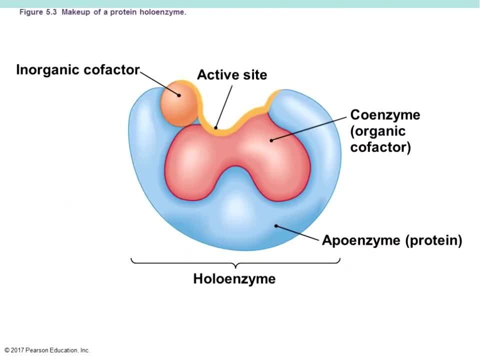 that exception to the rule that all enzymes are proteins. So here we have a pretty hollow enzyme, because it has the apple enzyme, the protein portion of it, and then you have this cofactor, which is the organic cofactor, and what it's going to build is that you have this active site here. So this 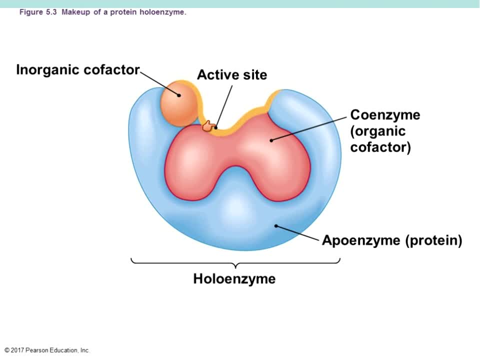 inorganic cofactor helps to build this active site. The active site is important because this is where the magic happens, So this is where all the stuff is going to happen is in the active site. If a substrate or a thing to be worked on by the enzyme does not fit this active 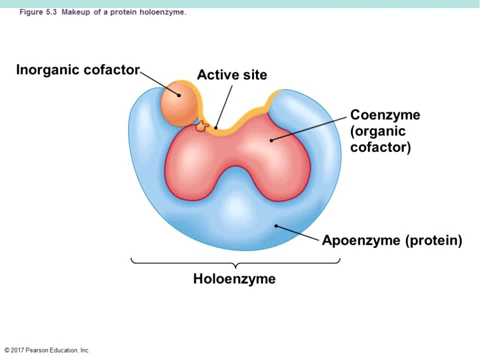 site then that thing to be worked on. AKA, the substrate is not going to be broken apart or built together, So it's important that we have a lock and key sort of matching that happens between the enzyme and the substrate in order for the enzyme to do. 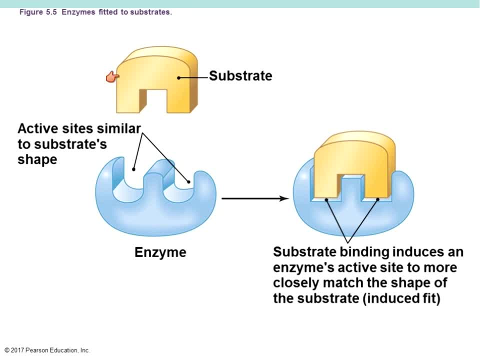 its job. So here we have our substrate. An easy way to just define a substrate is that it's just a thing that's going to be worked on by the enzyme. We're not going to say whether it's going to be built up or broken down. We're just going to say 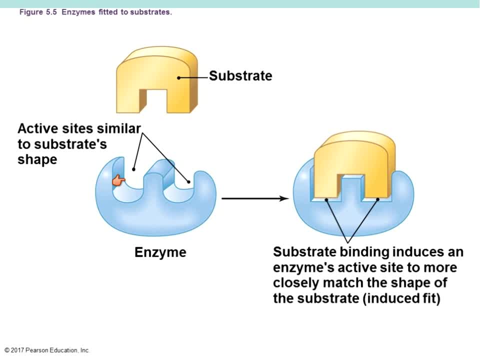 thing that's going to be worked on. so this enzyme has an active site and that active site is only going to fit this particular type of substrate. if it does not fit that substrate, then the enzyme can't work on that substrate. so the substrate binding induces an enzyme active site to more closely match that. 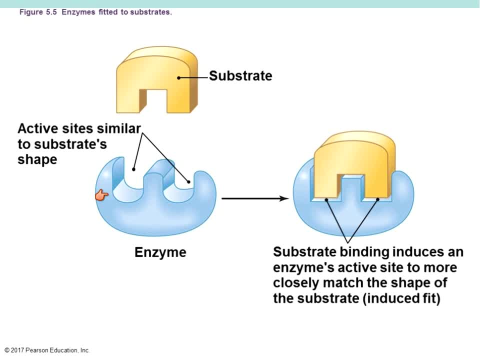 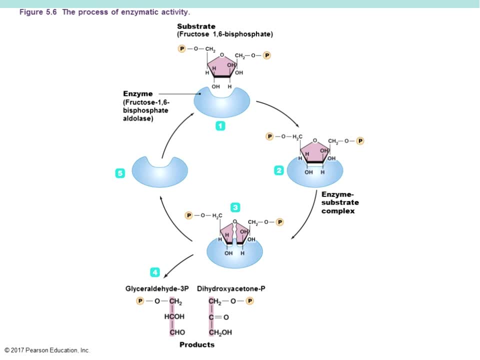 so this is what we considered a sort of an induced fit model, where it looks very similar to the active site and it's similar enough that we could get something to take place. so here is a pretty picture of an example of enzymatic activity as it refers to glycolysis. so before we're just looking 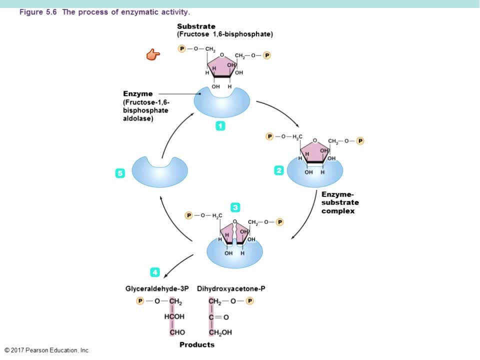 at like blocks and blobs. now we have a specific substrate- fructose 1, 6- biphosphate- and we have a specific enzyme- fructose 1, 6 biphosphate- aldolase- and so notice that the same principle still apply. we just put fancy. 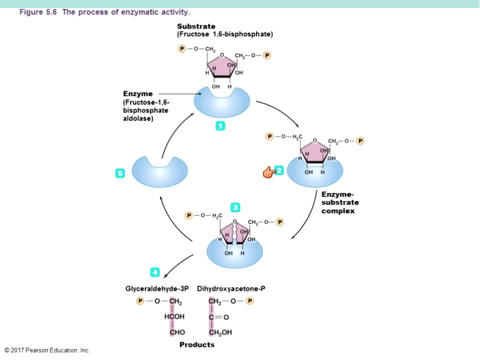 scientific names on it, that this is a specific substrate and that this is a substrate. it's going to fit into this active site. once the substrate fits into the active site, we call this whole combination an enzyme substrate complex. it's not all that difficult: we have an enzyme, we have a substrate substrate. 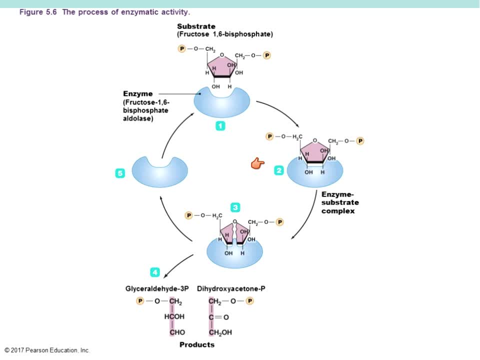 we are going to call the whole thing a complex. then, once we have our enzymatic activity, we can break it down into g3p and dihydroxy acid, lp. so we have these two products that come out of this. notice that only the substrate has been. 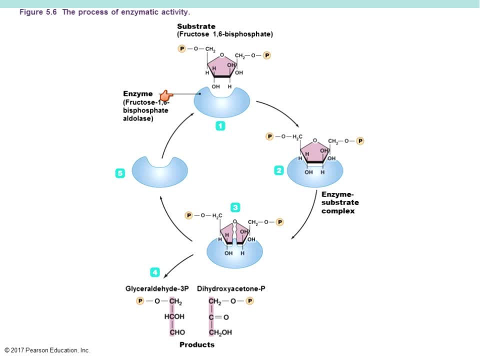 changed, the enzyme itself is unchanged, so then it can break down another fructose, 1,6-phosphate, into these two products, And this is an example of enzymatic activity that happens in one of the, in the first step of three of metabolism or cellular respiration, and this is glycolysis, or a step in glycolysis. 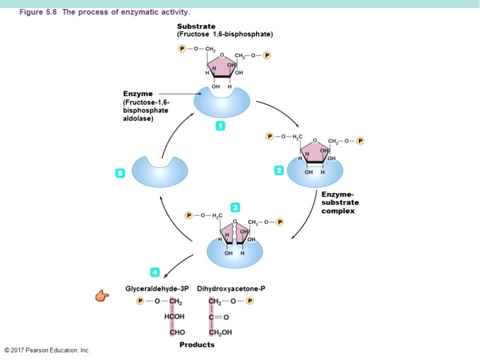 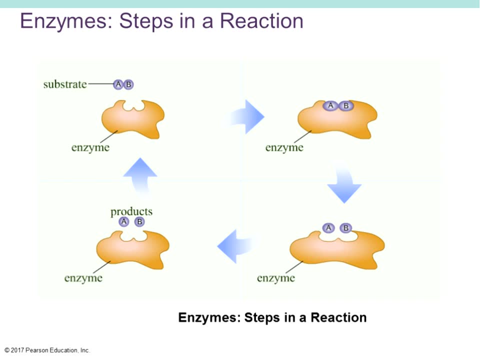 Glycolysis itself is a much, much more elaborate process, but this is just an example of enzymatic activity. So once again, I'm not going to really talk on this. I'm going to let you guys kind of investigate and see what goes on, because it's the same thing that we saw on the previous. 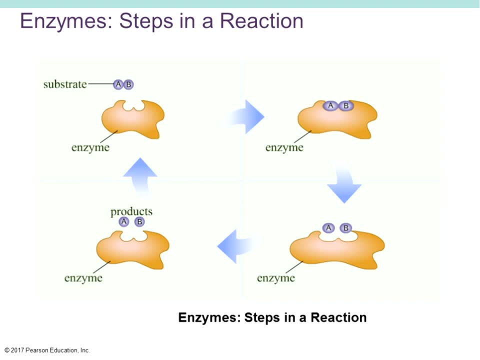 two slides so see if you can kind of think your way through it and I will come back. All right, so we have our substrate, broken down by our enzymes, fit into our active cell site from the enzyme substrate complex, and then these products are the only thing that 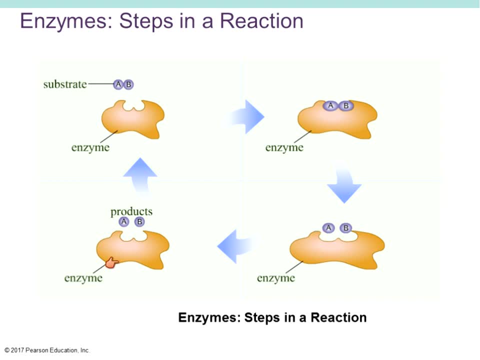 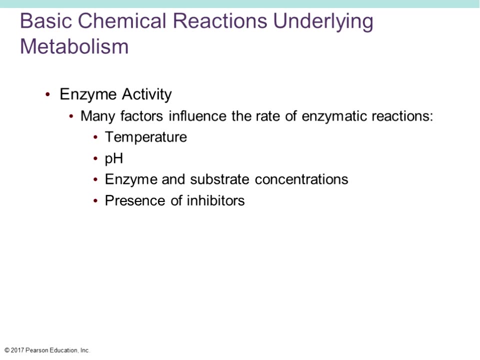 are changed, They're released from the enzyme and then the enzyme is going to be unchanged to do its thing again. So there are some factors that influence enzyme activity, and one of which you're probably already familiar with: the active site. So if the substrate doesn't fit the active site, then the enzyme's not going to do its. 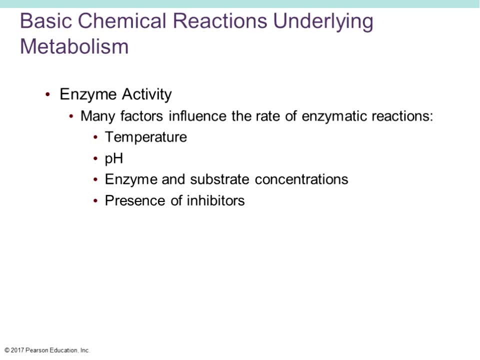 thing. Other things that can affect All right. Other factors that can affect enzymatic activity would be things like temperature. Temperature and pH can do something called denaturation. They can cause the enzyme to lose its shape. If the enzyme loses its shape or its form, it's also going to lose its function. 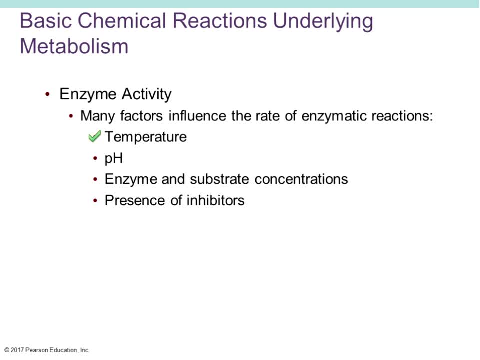 So if the temperature at which that enzyme is in, if the temperature's not quite right, if it's not the optimal temperature for that enzyme to function, or the pH is not optimal, then the enzyme can unfold and lose its shape. So therefore, if the active site is not configured the way that it should be, because of denaturation, 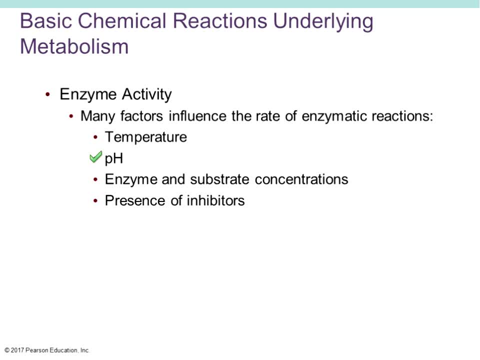 as a result of pH change or temperature change, then that enzyme's not going to work like we want it to. Other things that affect enzymatic activity are enzyme and substrate concentrations. So if we At some point throwing more substrate into the mix is not going to increase enzymatic, 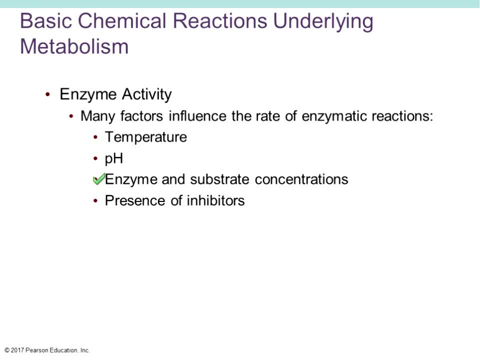 activity because that enzyme can only turn over or work so quickly. So, as a result, If you have a too high of a concentration of substrate in ratio or relation to the enzyme, then those substrates aren't going to be worked on in any faster because the enzyme can only 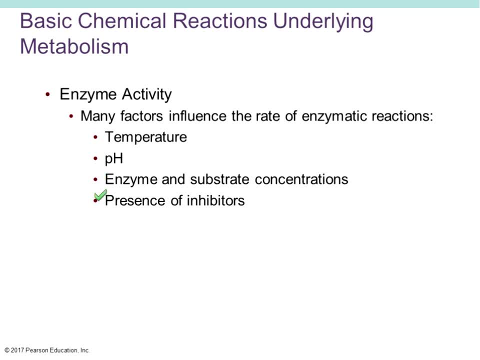 work so fast. And then finally the presence of inhibitors, And conversely the same way. if you have lots of enzymes and very few substrates, then you're going to have those substrates broken down very quickly. So inhibitors can either be competitive or non-competitive, and when something is inhibited, 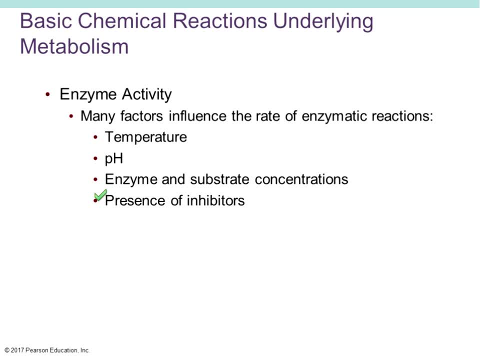 it means it's prevented from doing its thing. So enzymatic inhibitors will prevent an enzyme from working on its substrate. So either competitively, by fitting the active sites themselves, or non-competitively, by just fitting a site outside of the active site, but it causes the active site to change its 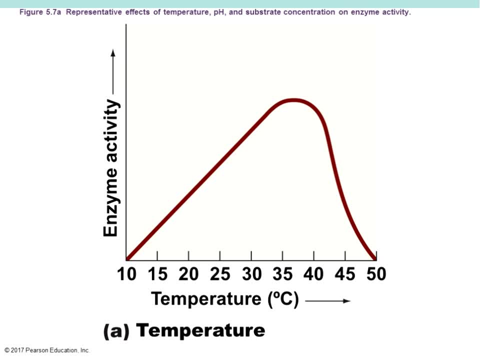 shape. So temperature: notice that for this particular enzyme, that the optimal temperature is right around here, I would say about 37 degrees Celsius, which happens to be the exact temperature that we're talking about. So that's the temperature. It's the exact same temperature as your body temperature for most of us. 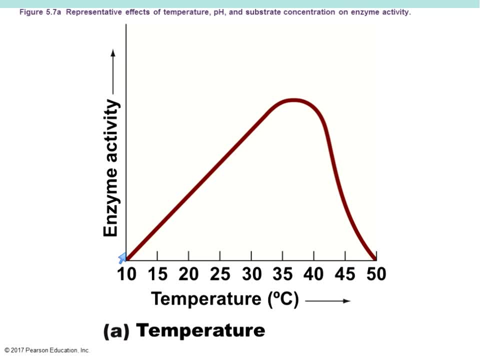 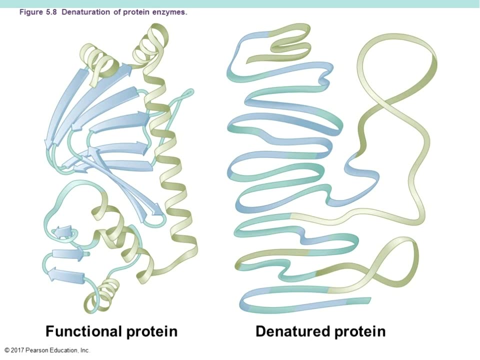 So anything too much higher than that or much lower is going to reduce the amount of enzymatic activity. If it's right there at 37 or around 37, then it's going to have the most or optimal enzymatic activity. The process of denaturation that we talked about. this is just the protein losing its 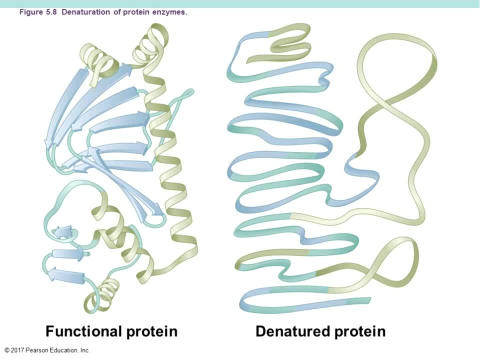 shape And, remember, most of the enzymes we're talking about are protein And if it loses its form, it's going to lose its shape. If it loses its form, it loses its function. So if this guy here is the active site, then where on earth is the active site over here? 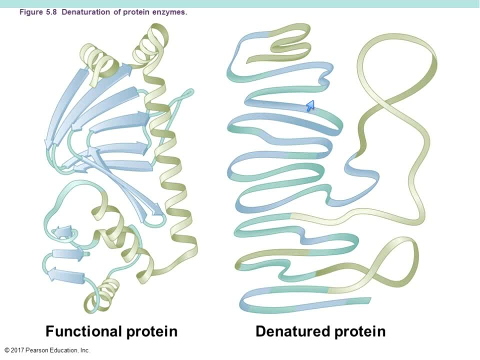 It doesn't really fit very well. So, too high a temperature, too low a temperature, anything outside of its optimal range, And keep in mind that all enzymes have the same optimal range for temperature. Some might like a much higher temperature as its optimal range. 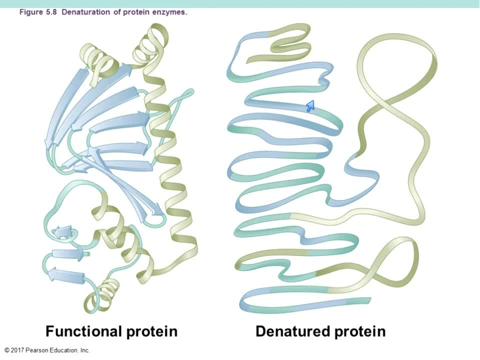 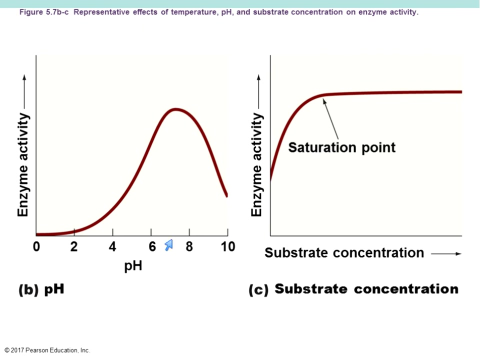 Some might like a much lower pH or higher pH. So these ideas of temperature and pH being optimal. The optimal temperature is the optimal range. The optimal temperature or optimal pH can change just depending upon where that enzyme is normally found. So for pH here looks like about 7.. 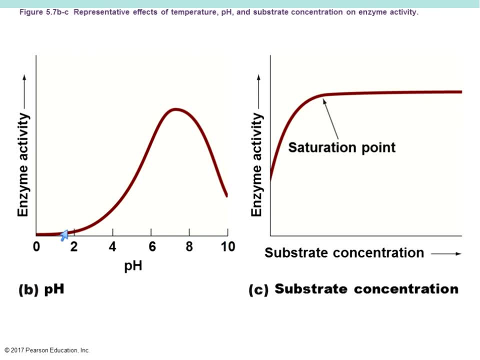 That's where we're going to have the highest amount of activity. Anything much higher than that or lower than that is going to reduce enzymatic activity And then substrate concentration. That notice that our enzymatic activity will increase as we add more substrate. 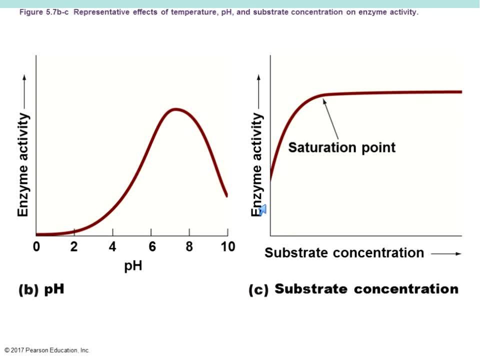 So substrate concentrations increasing on this end. So as we add more substrate, The enzymatic activity will increase. So that's where we're going to have the highest amount of activity. It will increase until we get to a point and we call that our saturation point. 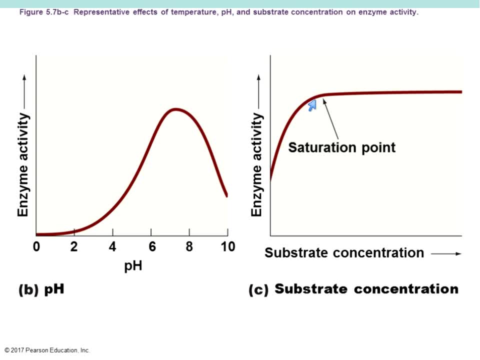 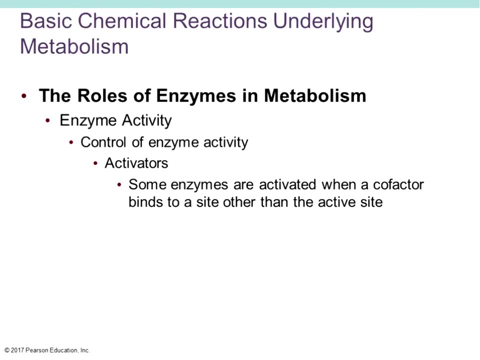 At this point the enzymes are saturated and no matter how much more substrate you put in there, they're only going to be able to work so fast and turn over the substrate into the product that it needs to be so quickly. So the roles of enzyme in metabolism: control of enzyme activities, activators sometimes. 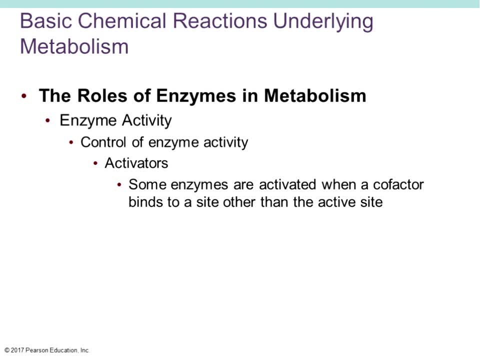 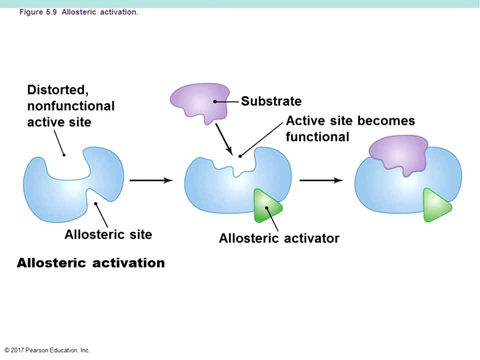 are activated by a co-factor that will bind to a site other than the active site And if it changes the active site we will consider that a non-competitive inhibitor. We call that site outside of the active site the allosteric site. 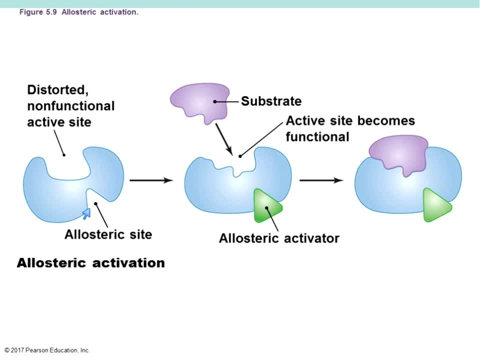 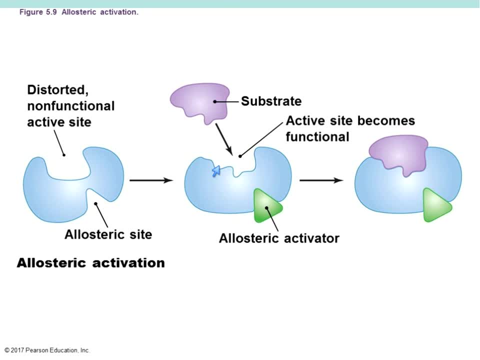 We can have some co-factor, We can have some co-factor, We can have some co-factor, We can also have some that act as activators And that now we've had the active site change so that it can fit the substrate and the enzyme. 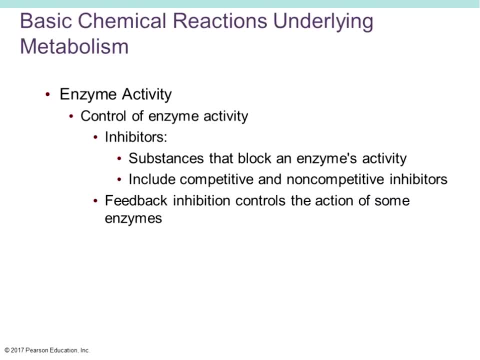 becomes more functional. As I said before, we have inhibitors, We have non-competitive and we have competitive inhibitors. Non-competitive inhibitors would fit that allosteric site that we just saw on the previous slide, And the reason that we would want inhibition to take place is so that we can control the. 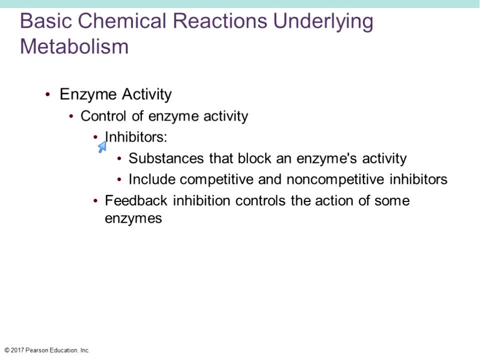 we can control the action of those enzymes. so we don't. if there's, if there's only so much of a substrate to be broken down, we have enough of the product. then we don't need to continue to break down and build more products. so that's a. 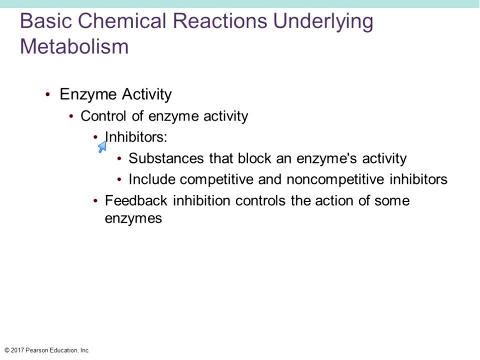 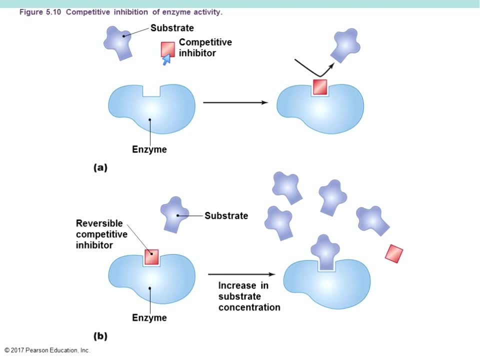 waste of energy. so they're meant to kind of regulate the activity of metabolism. so here we have our substrate and our competitive inhibitor. notice that they both kind of look the same and match that active site. so at this point if the competitive inhibitor was to get into the active site and they have out. 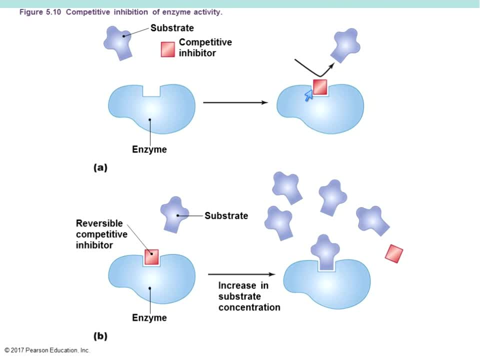 competed the substrate. so this competitive inhibitor is going to actually keep this enzyme from doing its thing, from breaking anything else down. it just caused it to stop working. so we have here that reversible competitive inhibitor that, if it were to be removed, and we increase the substrate concentration if there are more of the substrates than there are of the inhibitors. 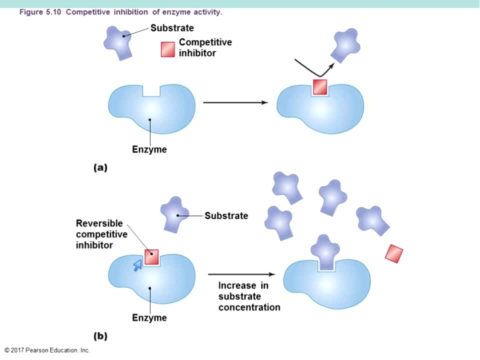 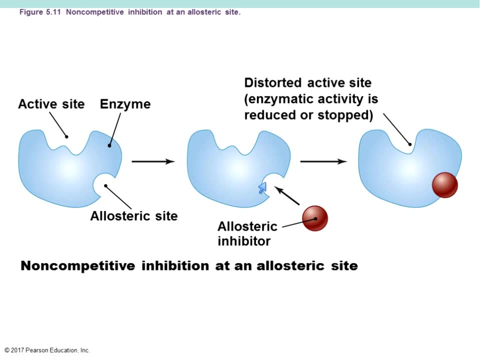 then that would allow the enzyme to work again. So non-competitive inhibitors notice also the allosteric site and much of the same way as those cofactors fit in the allosteric site and it caused the active site to change. except this time when we changed the active site, we distorted it so that enzymatic activity. 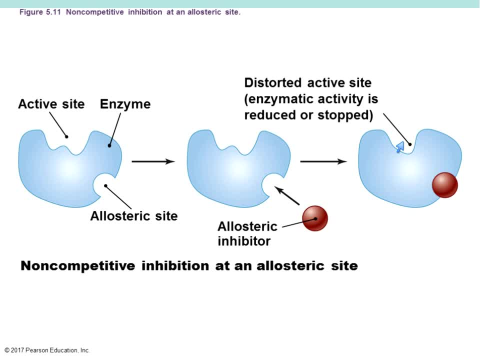 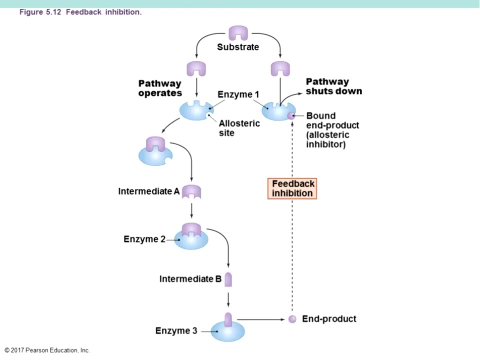 had stopped, as opposed to enhancing enzymatic activity with those cofactors. So this would be an example of non-competitive inhibition doesn't out-compete the substrate for the active site, it just changes the active site. And so here's a picture of that feedback inhibition here. 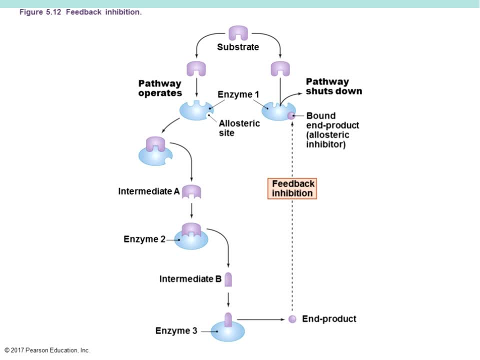 So if we have our different end products that come out of here. so what we're working with is that we have our enzyme that's doing its thing, so we have our enzyme 1, the substrate gets broken down and we continue. as long as there's no product, then we continue to. 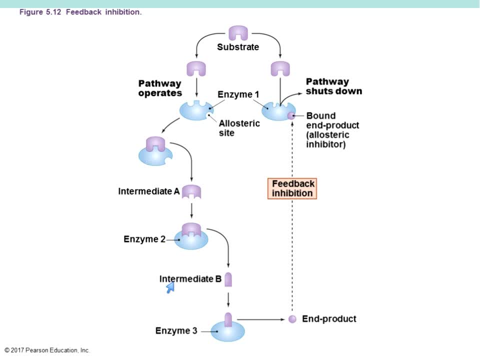 break down. we get our end products, our intermediates, and then we get this end product. Now we'll keep on going through this process, because at this point we have more substrate than we have end products. so we'll keep on going through this process until we have a 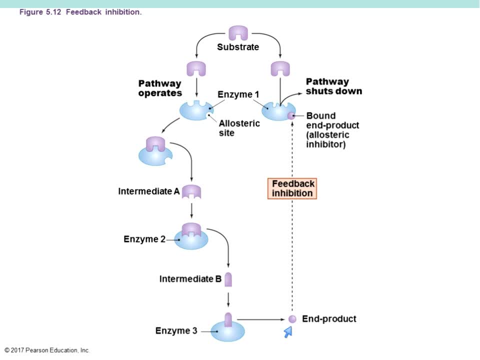 new substrate. So we have enough of this end product that's made that we say: okay, we don't need this enzyme to work anymore. So because we don't need this enzyme to work anymore, it will fit the allosteric site of 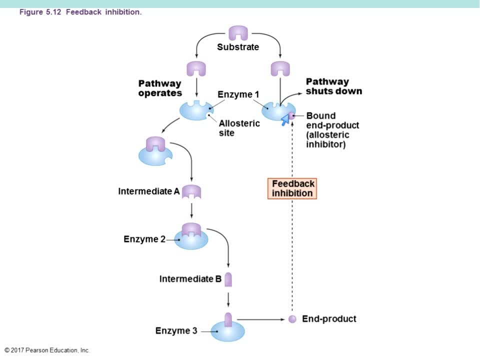 the very first enzyme that was at work here. So because it fit that allosteric site, it caused the active site to change and it inhibited the enzyme from working. So it's basically putting the brakes on the product itself. it's putting the brakes on 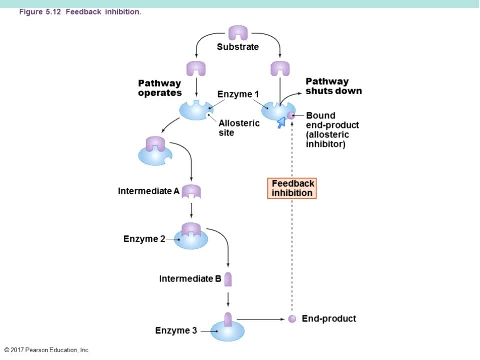 the activity of this enzyme, And what type of Inhibitor is this? competitive or non-competitive? Non-competitive inhibitor? because it's bound to an allosteric site, a site outside of the active site, but it caused the active site to change its shape and it stopped the enzyme. 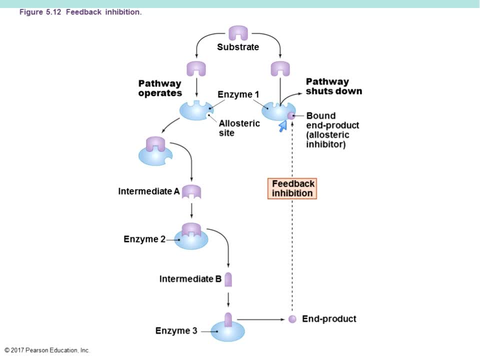 from working. Why on earth would we want to do this? Well, if we have enough of this end product, what sense does it make to keep having this protein or this enzyme go through this advancing process? So the first type of catabolism that we're going to talk about, and we'll talk briefly- 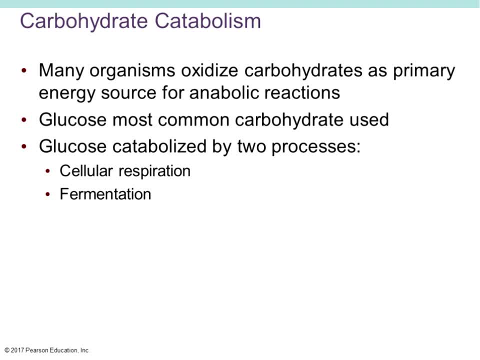 about lipid and protein catabolism is carbohydrate catabolism. It's the most well-understood type of catabolism and it's pretty universal. at least some parts of it are universal, like glycolysis basically happens in everything. 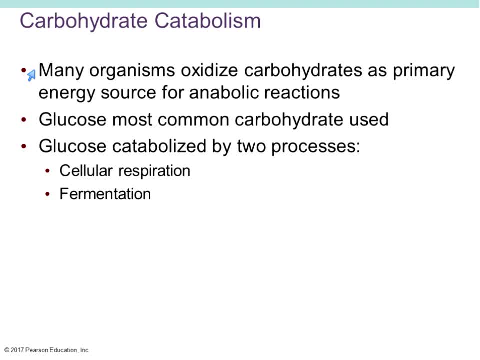 Lots of different organisms will oxidize carbohydrates as their primary energy source. Glucose is going to be that most common carbohydrate that's used. Glucose can be catabolized or broken down by two different processes: Cellular respiration and fermentation. So that's why we say that carbohydrate catabolism is pretty universal and it is definitely 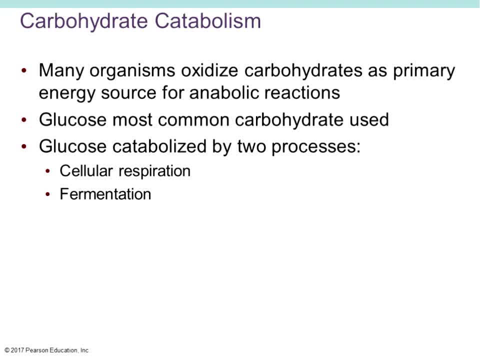 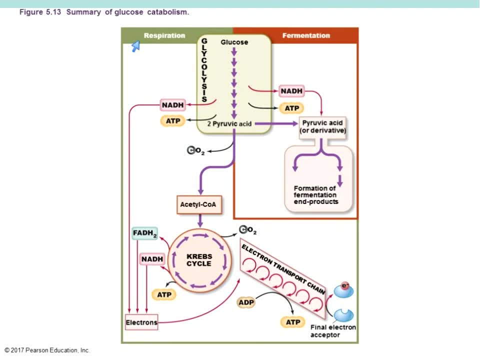 the most well-understood type of catabolism. So a summary of glucose catabolism: remember those two different types that we had. We had respiration and we had fermentation In a respiration. you can probably just already look at it: everything in the green box is 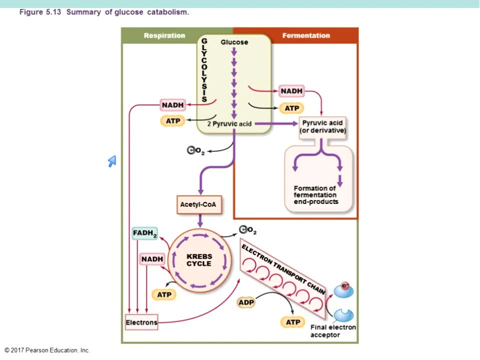 considered part of respiration or part of the respiration step, But it is pretty intense. So there's glycolysis that takes place, then we have the Krebs cycle in step two and then the electron transport chain is the final step. 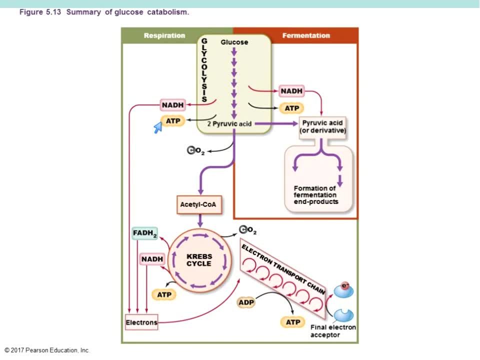 Even though it's pretty complex, the good news is we're going to get ATP that comes out of three different steps, So we're going to make more ATP in this process. However, it's a longer, more complex process and it's going to have different requirements. 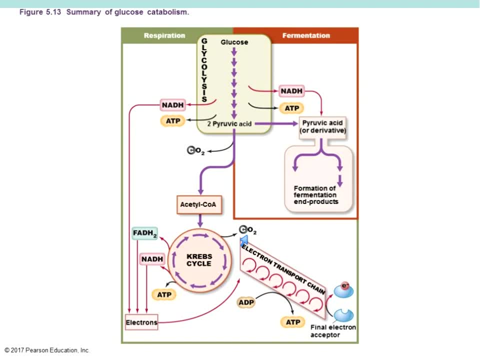 One of those requirements may be. you know you're going to have a lot of energy, you're going to need oxygen, So you might need oxygen as a requirement, or different types of molecules could be a requirement for it, And we'll discuss those later on in the next session. 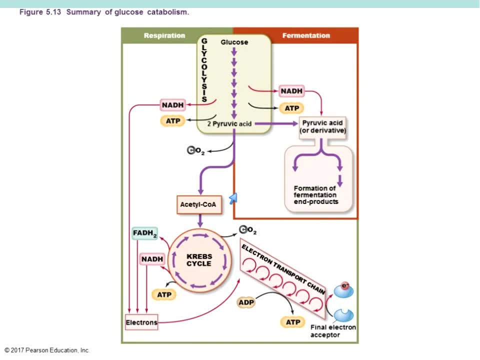 And then we have fermentation. Fermentation is everything in the orange box. It's a lot simpler process than respiration, but it doesn't. it's not going to give you ATP from as many different places as we saw with respiration, But what we do notice is this is a very complex process. 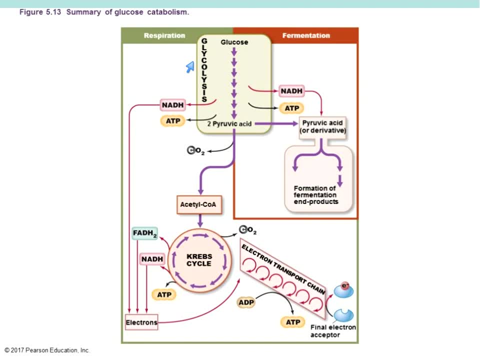 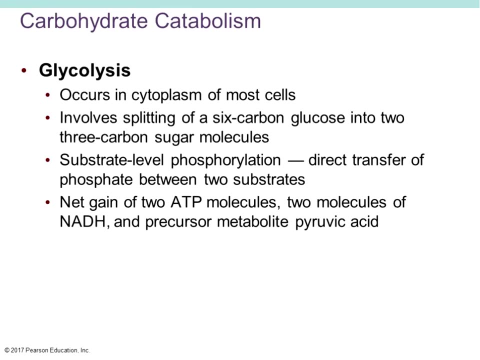 It's a step of glycolysis. It's shared between both respiration and fermentation. So glycolysis is the first step of both fermentation and for respiration. Glycolysis, where it happens, is it's going to take place in the cytoplasm of most cells. 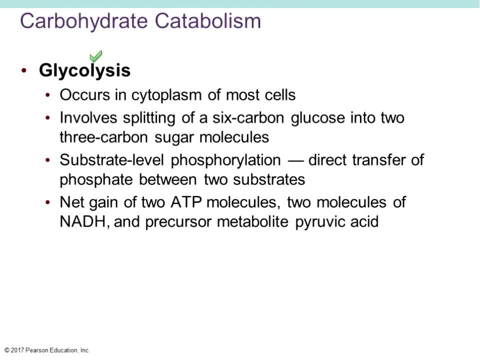 And the process of glycolysis- glycose glucose lysis- breakdown- is going to involve breaking down glucose, that's six-carbon sugar, into two-carbon glucose. So glycolysis is the first step of both fermentation and for respiration. 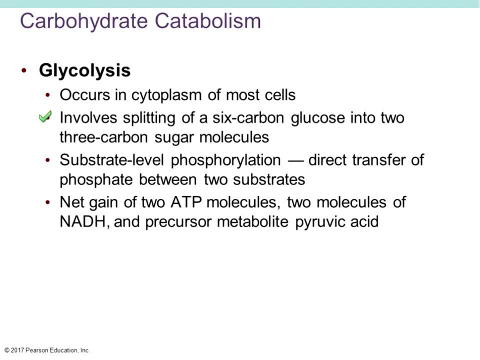 Glycolysis is going to take place in the cytoplasm of most cells And it's been medicated throughout the body for 10 toolboxes that usually take up to 23 carbon sugar molecules. During this process of glycolysis we're going to have some ATP made and we're going to 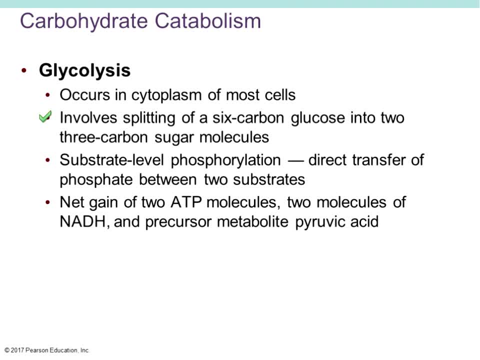 and it's going to be made through what we call substrate-level phosphorylation, where we're going to directly transfer that phosphate function or group between two different substances At the end of glycolysis. what our net gain, what comes out of this process, is we're going 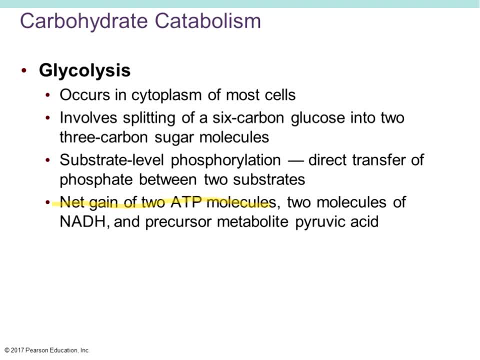 to get two ATP molecules. notice- I'm highlighting this because it's very important- We get two ATP molecules, two molecules of NADH and these NADH molecules. these are our electron carriers, So they're going to always take their hydrogen and electron directly to the electron transport. 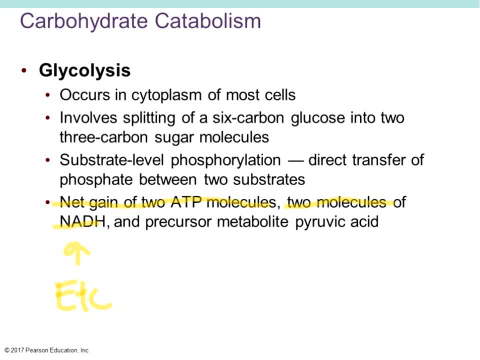 chain, if this glycolysis is going into, is part of cellular respiration. If it is part of fermentation, it's still going to carry those hydrogens and electrons but it goes to a different, through a different process to get this fermentation to start.